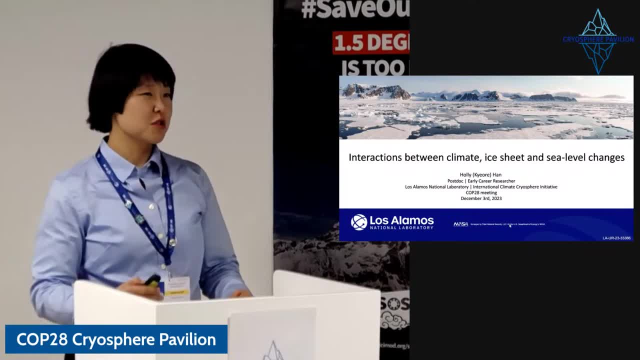 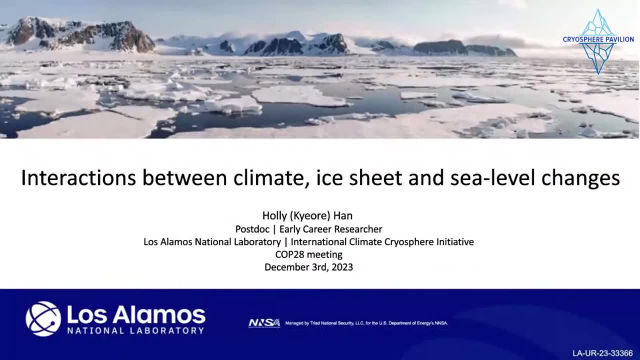 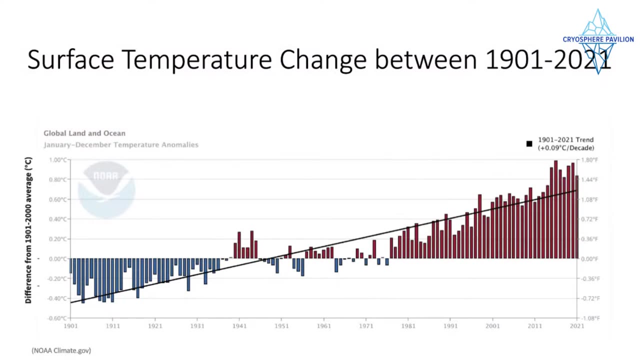 So today I'll tell you about my research, but also cover a higher level of climate interactions between interactions between ice sheet, climate and sea level changes. The slide shows the surface temperature change between the 1901 to 2021.. It is actually showing. 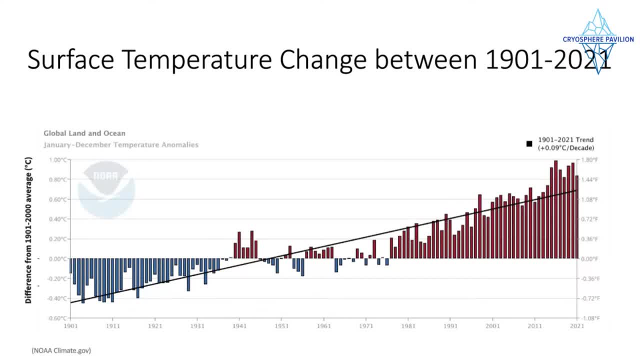 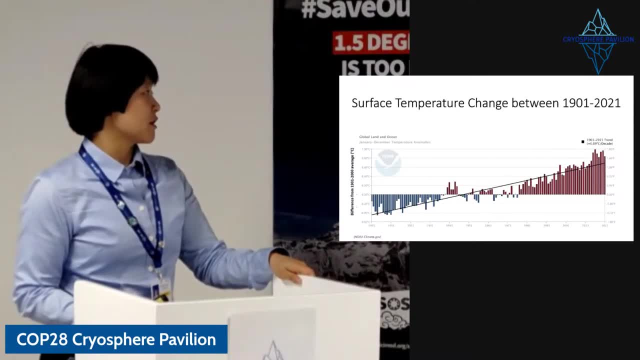 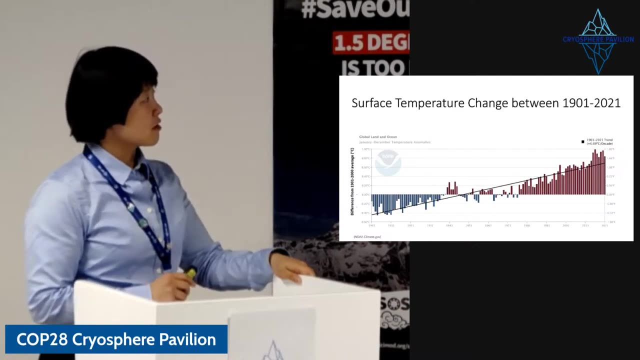 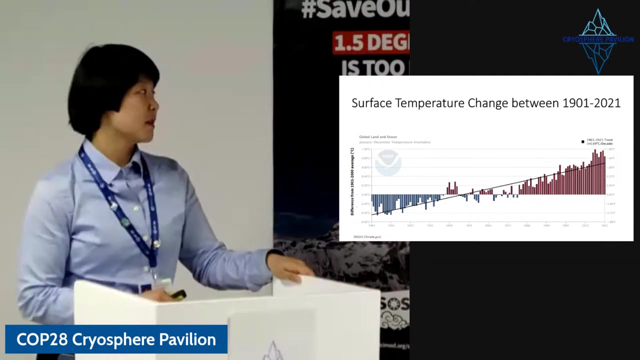 the difference from climate temperature, global temperature average for respective years relative to the average value between the 20 1981 to 2000.. And you can see that the global temperature actually has been rising at the rate of 0.09 Celsius per decade, And so this warming was clearly due to. 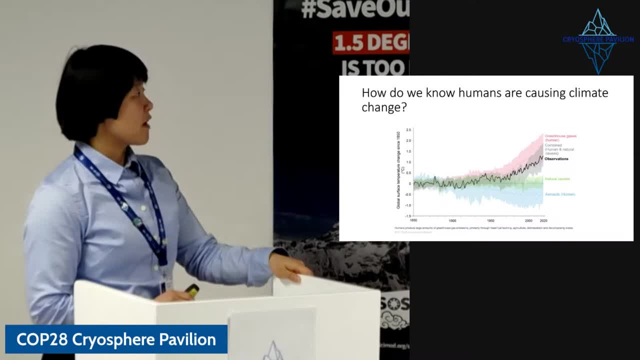 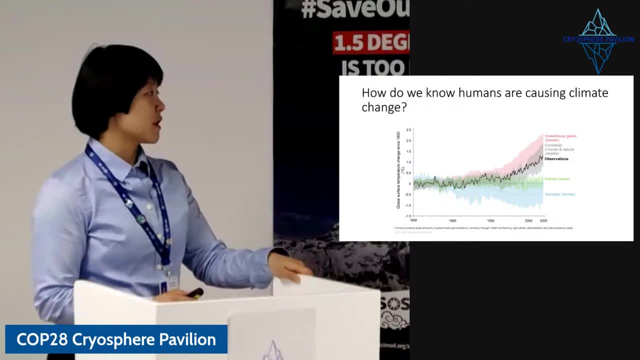 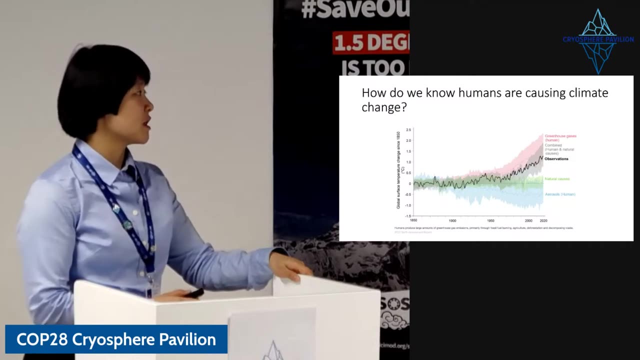 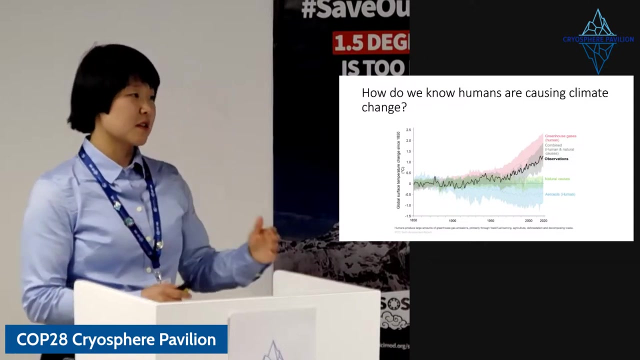 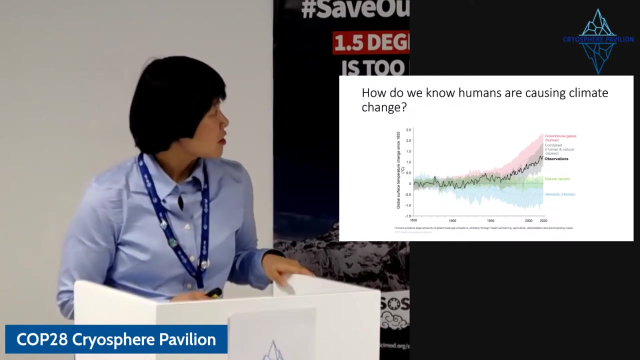 a lot of components And, however, the black line here that shows the observations of global surface temperature since 1950, can only be explained when we incorporate the greenhouse gases emitted by human activities, shown in red, and the natural causes shown in green and aerosols due to human activities that reflect sunlight off in the air, shown in blue, and the gray color showing the combined natural causes. that is actually matching the blue curve, the observation lines. 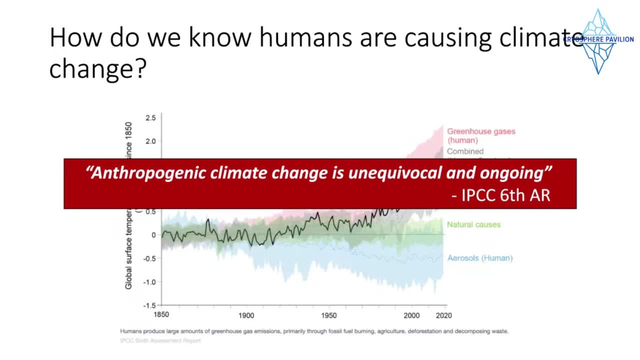 So in the latest IPCC report, sixth report, said that anthropogenic climate changes is unequivocal and ongoing. So there is no question as to the reason for the current rate of climate change is due to climate, human activities. So what is the problem with recent climate change trend? 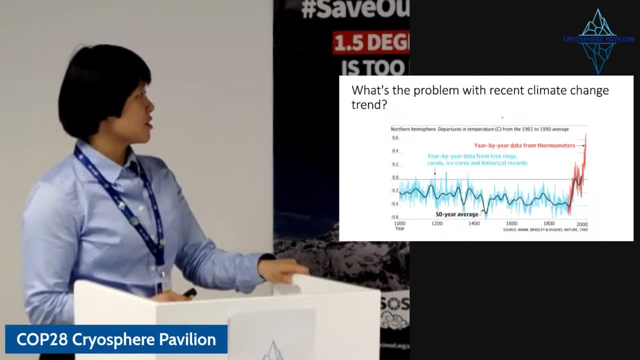 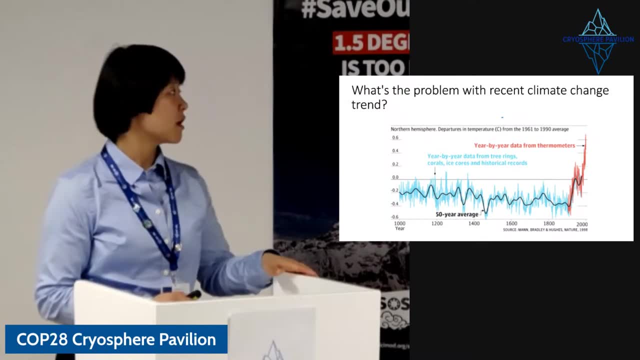 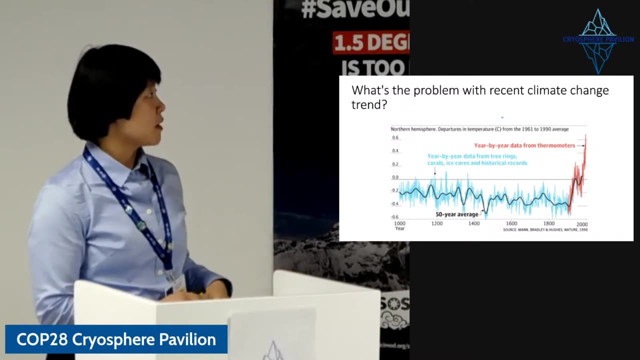 This plot is showing the temperature changes through the last thousand years- about thousand years- And this is also famously called the hockey stick plot by Michael Mann et al- And it's showing the temperature changes in the northern hemisphere compared to the average value between average taken between 1961 to 1990.. 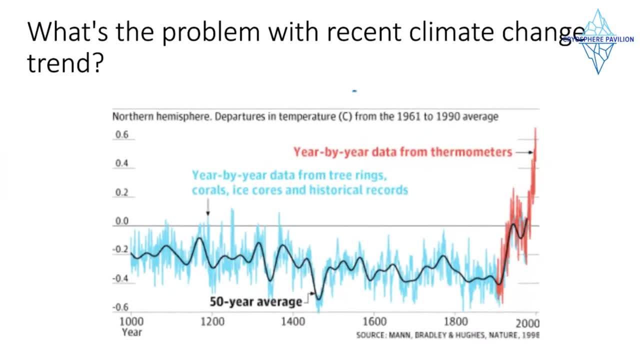 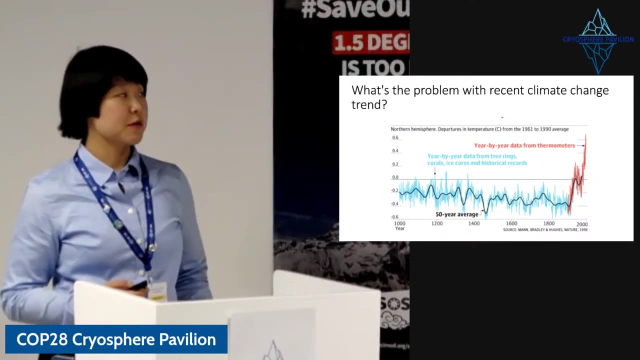 And you can really see that in the blue curve, The temperature changes recorded in the blue curve. So the temperature changes in the natural resources like tree rings, corals, ice cores and historical records have been quite flat compared to the rate we've been experiencing in the past decades. 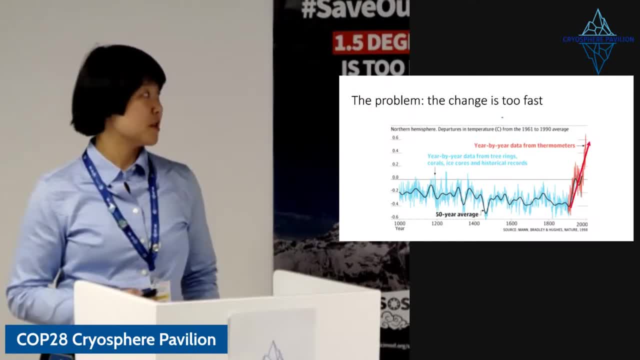 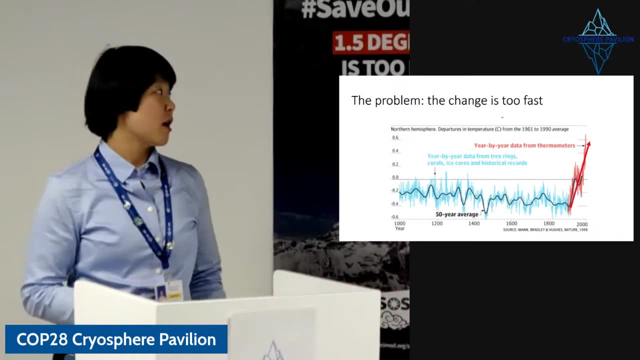 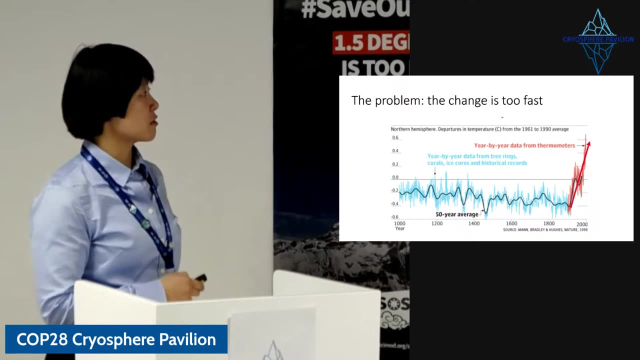 And so the problem is that this change has been is too fast. Obviously, there has been changes through the last thousand years due to natural causes, But because of the human activities we are still in a state of crisis are actually accelerating this rate of climate change. 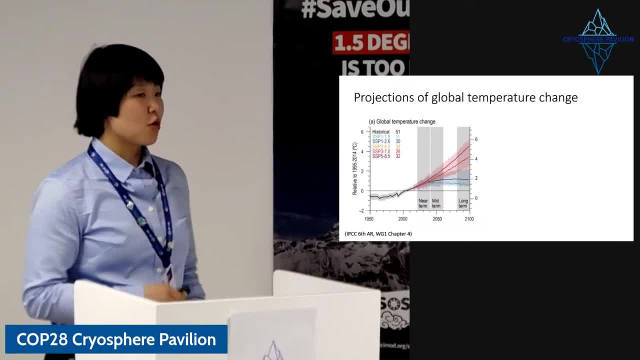 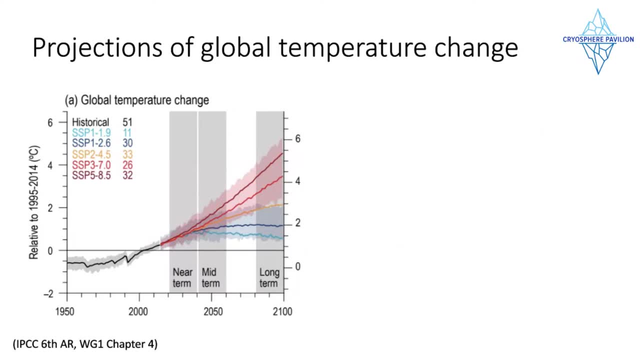 or global temperature warming. So going forward, what is going to happen, is something that everyone is curious about, And so here the plot is showing the projections of global temperature change through the 21st century, And all the values are comparison relative to the average taken between year 1995 and year 2014.. 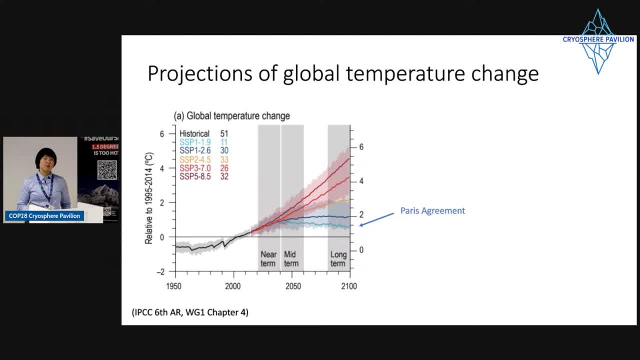 And this blue line is what we agreed upon in the Paris Agreement. So this is about 1.5 degrees Celsius warming by the end of the century, And then as you go, higher and higher in number, it represents that the forcing is stronger and warming is stronger. 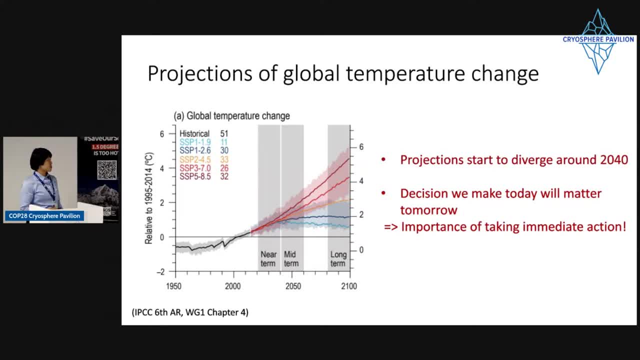 So we can see that the projections really starts to diverge around year 2040, that's about in 20 years time, And it implies that the decision that we make today will really matter tomorrow, And it really also implies that the importance of taking immediate action, 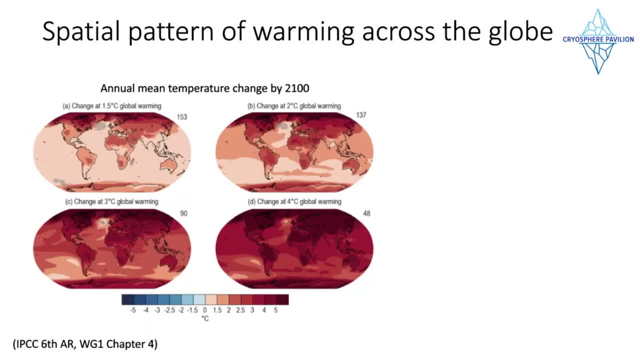 So what does the spatial pattern of warming across the globe look like? taking these different scenarios, these line scenarios, into spatial patterns? On the first right top is showing the annual mean temperature change by the end of the 21st century, When we take the path of warming the globe by 1.5 degrees. 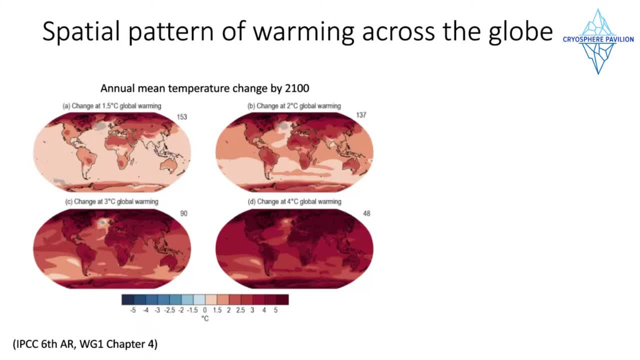 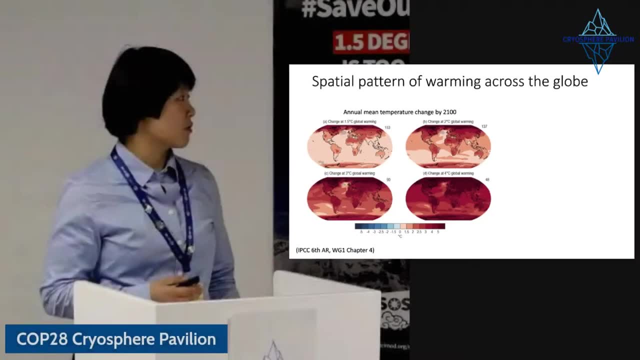 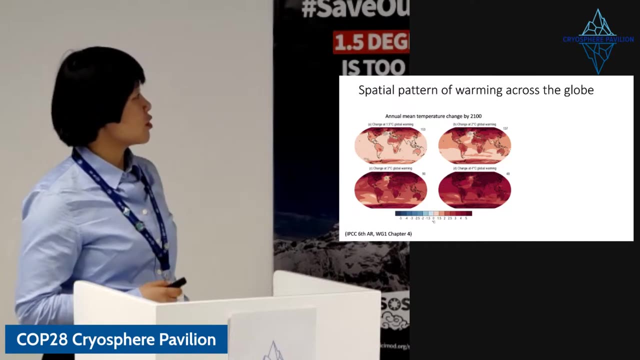 And on the top right is changing two degrees and the left bottom is changing three degrees And the left right bottom plot is the temperature projected when we in the scenario of four degrees of global warming. And we can see that in the first top two plots. 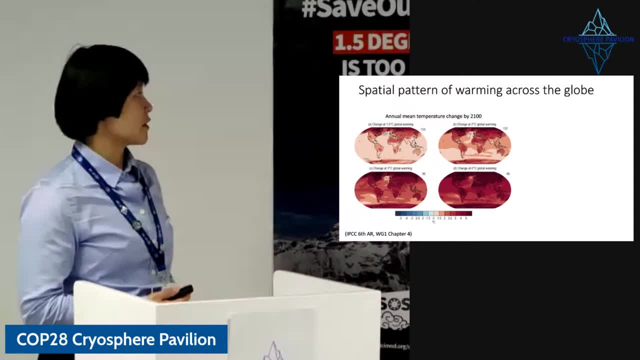 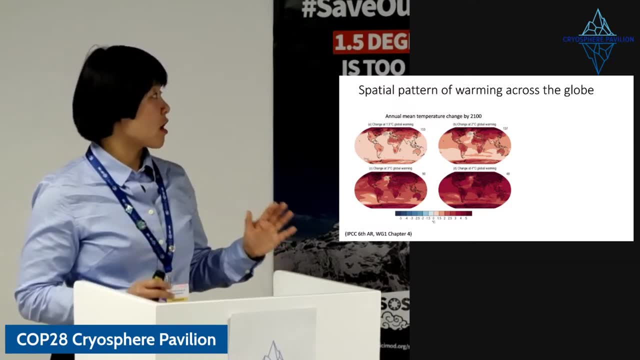 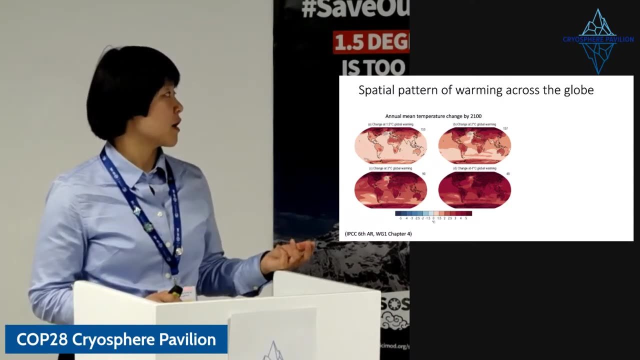 the Arctic regions are amplified due to the polar amplifications And so the average values. when it's mapped across the global- it's global coverage- you can really see that the red regions are going to experience a lot higher global warming compared to the average value. And at the bottom. when we go beyond three or four degrees, then almost the entire globe gets really, really red, experiencing higher than four to five degrees of warming. So looking at the difference between two degrees versus 1.5 degrees warming at the very top on the TOP, 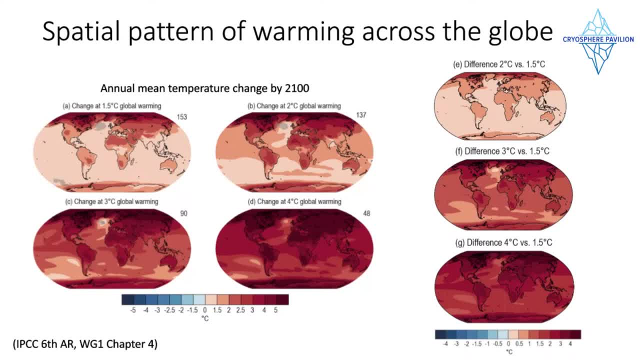 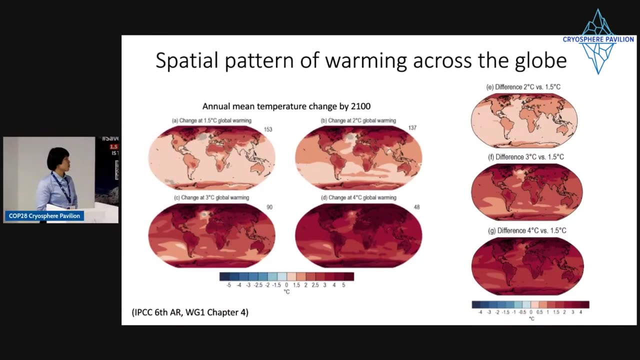 on the right hand side you can see that it's already pretty well. we're taking that only 0.5 degrees of difference globally average value. but when you look at the spatial pattern it's going to be a lot higher than 0.5 degrees. 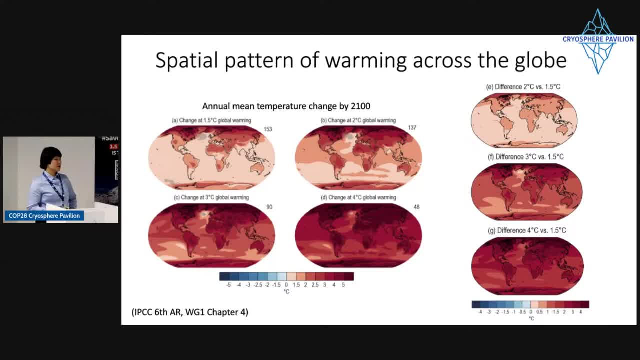 up to 1.5 or two degrees. So we always have to provide- think this globally average value in terms of spatially varying values, and more like a globally average value, rather than just thinking that this is only a small number that isn't going to cause. 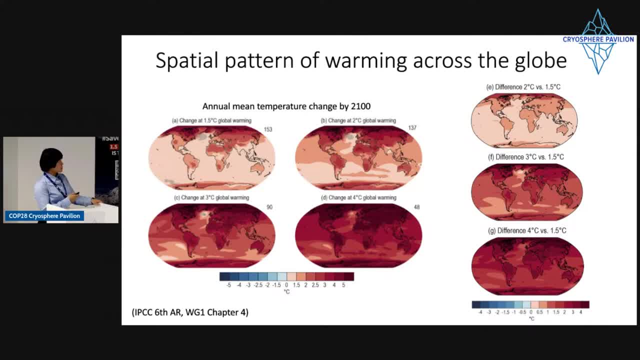 any trouble for us. and this difference plot obviously gets really red, gets redder and redder as you go um higher degrees. so at the bottom difference between four degrees warming scenario versus a 1.5 degree warming scenario, um the difference is going to reach more than 3.2.5. 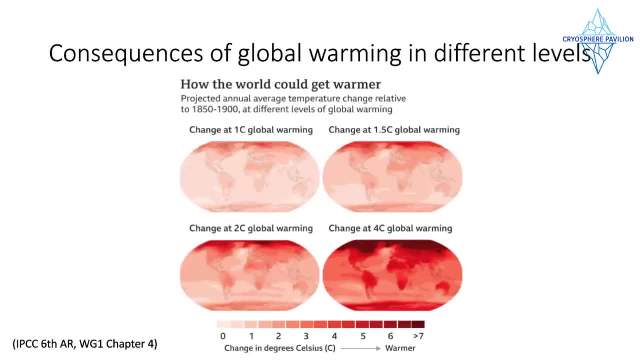 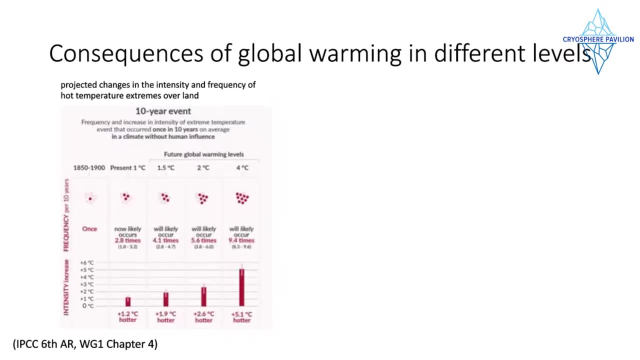 degrees. so what are the consequences of global warming in different levels? um, this is showing the pattern of global temperature by the end of the century and, as i saw before, and at the same time, we're going to have really more exacerbated climate events, for example, the 10-year event, which means that an event climate 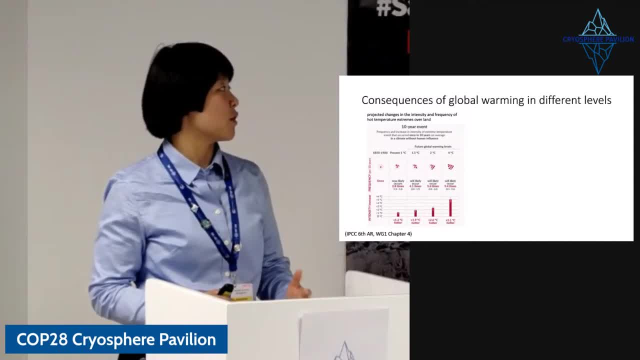 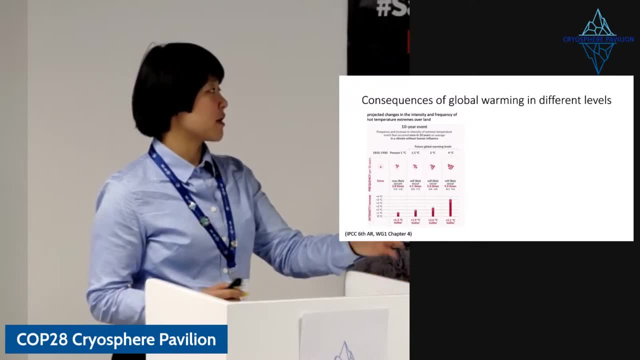 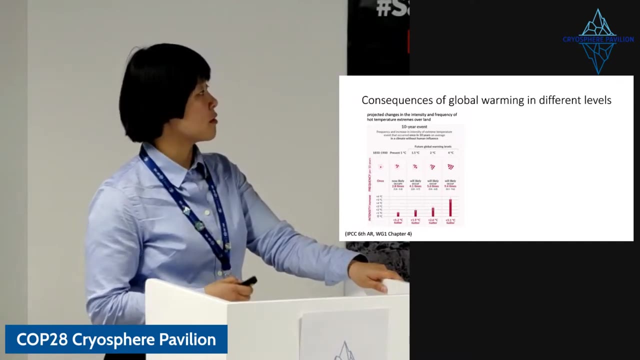 extreme event will would have would have happened once in 10 years during the in the pre-industrial climate. at present day, it is now likely uh happening at 2.8 times per 10 years and when? if you compare the projected differences between 1.5. 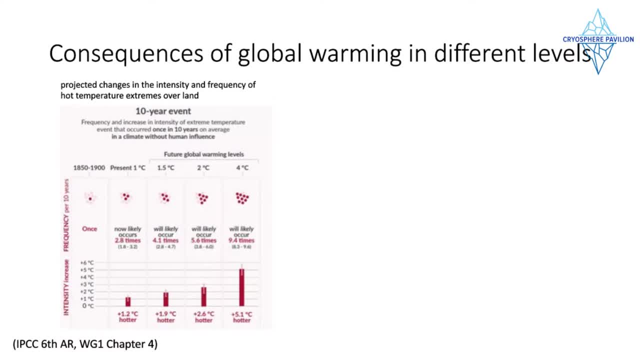 degrees roaming scenario versus two degrees, that is now jumping up to 4.1 times more and five times 5.6 times more respectively. and as for the 50-year event, again if you compare 1.5 degrees warming cereal versus 2.5 warming scenarios, 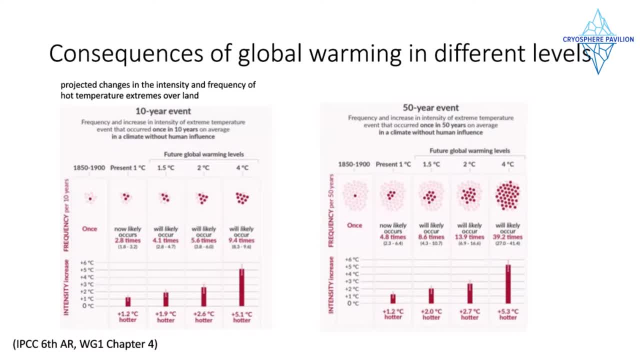 what used to happen every 50 years is going to happen 8.6 times and 11.12.9 times. so let's look at that and then we'll look at theever spending, that change contributing to global warming there there were a few interesting improvements. 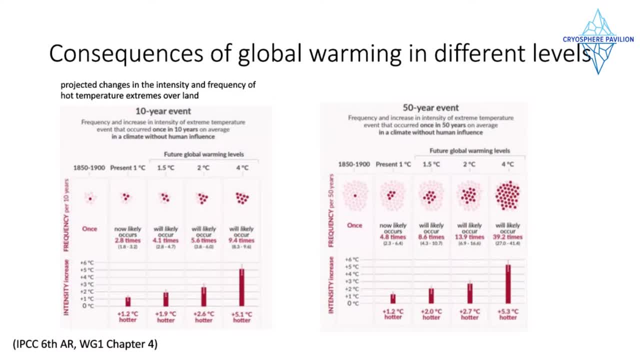 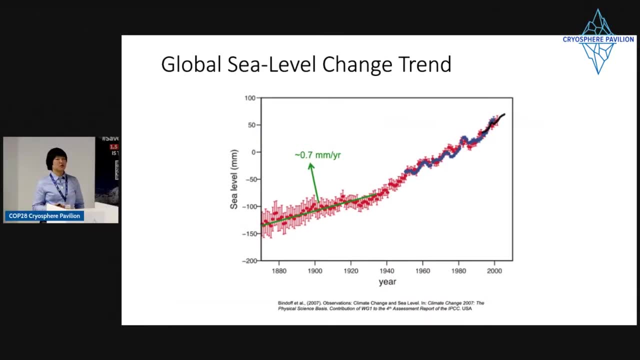 so, for example, especially on conservation of the environment, many people who were working in the forest hose was doing the same kind of research to provide some information from the sort offunds that we use to look at dish management as far as European farming is concerned. but change in the past. 21st, 21st century We had the tide gauge. records suggest that the sea level 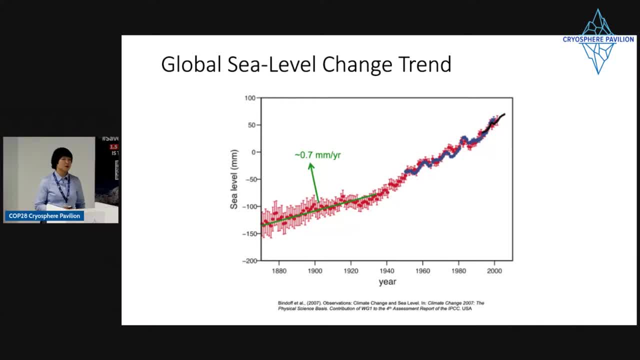 has been rising. sea level has been rising at 0.7 millimeters per year for the first part of the 21st century, 20th century- and at two millimeters per year at the mid to towards the end of the 20th century, And then right now we're seeing at the end of the 20th century. 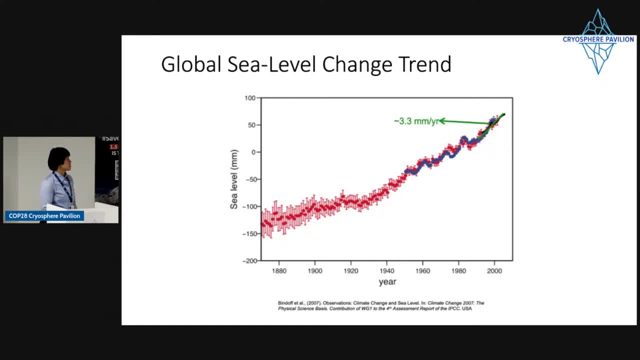 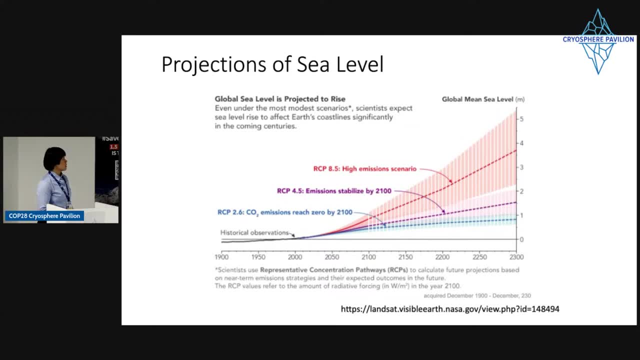 we've been seeing about 3.3 millimeters per year sea level rise rate. So the question is: what is going to happen in the future? So same as similar to projections of global temperature. this is projections of sea level in different scenarios And the green 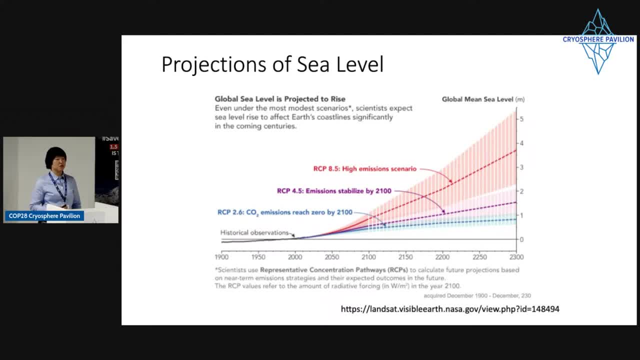 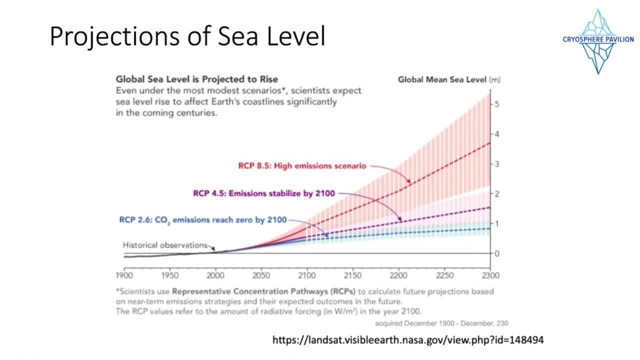 blue line RCP 2.6 scenario is where we keep the low emission as we've agreed upon during the Paris Agreement And, as you go, redder and redder sea level is going to increase more And the possibility of having experiencing dramatic sea level rise increases as well. 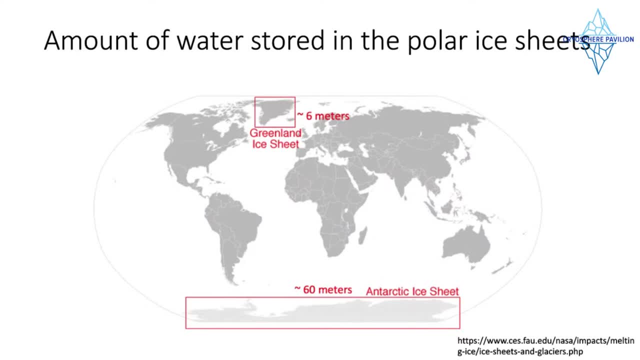 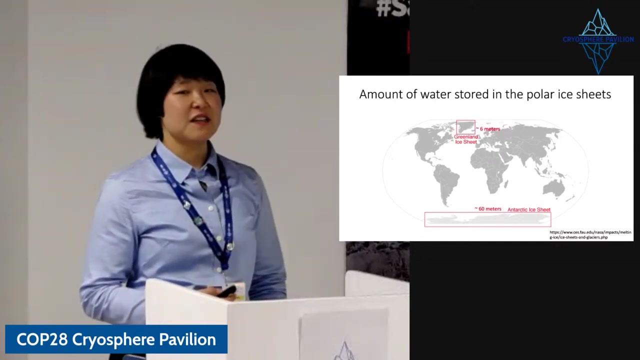 So where would the sources of this dramatic sea level change, or future sea level change, are mostly the polar ice sheets in Greenland and Antarctica. In Greenland there's about six meters equivalent sea level ice volume locked up, And in Antarctica there's about 87,, 87,, 80,- sorry, 57 and 58 meters of. 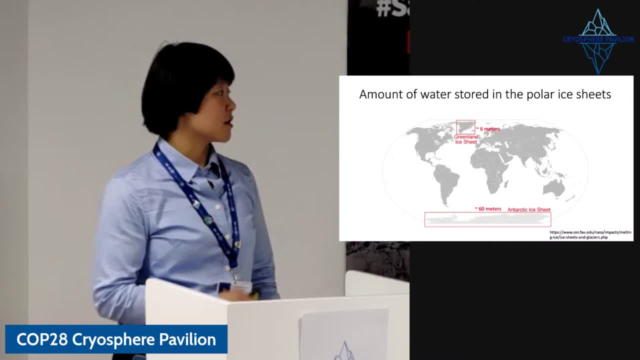 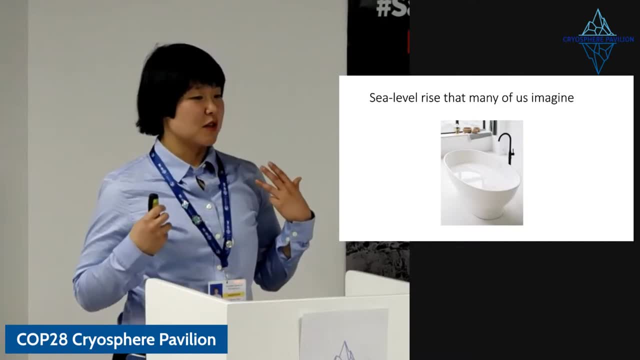 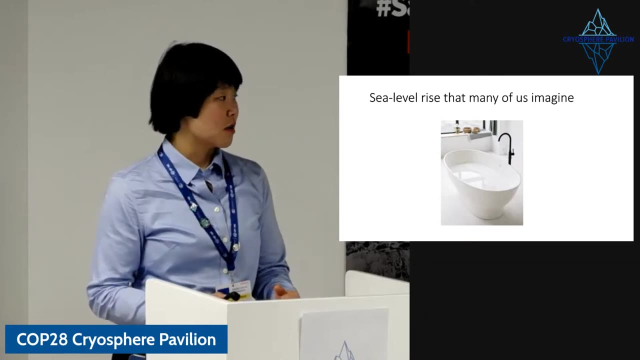 sea level equivalent ice volume locked up in Antarctica. So that's a pretty big amount of ice. And so what would happen when? when we melt these ice sheets, when these melt ice sheets start melting, our intuition, or our intuitive imagination, suggests that sea level will rise. 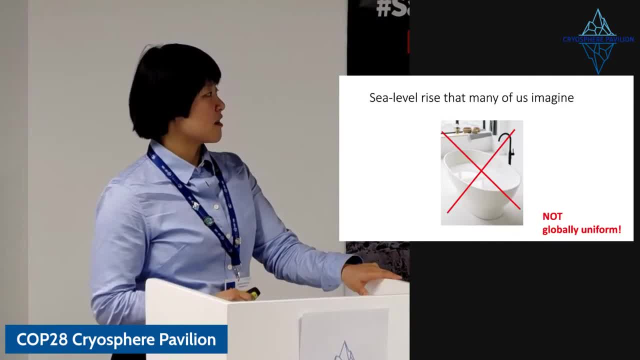 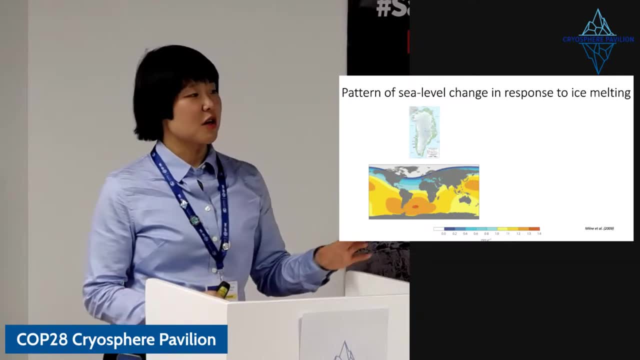 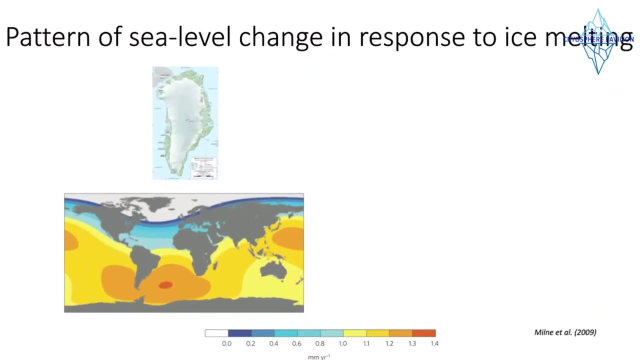 globally uniformly. But actually that's not true. Sea level actually changes. sea level change pattern is pretty complex. So for example, in the green and blue regions when Greenland ice sheet melts, the bottom part is what the pattern would look like. 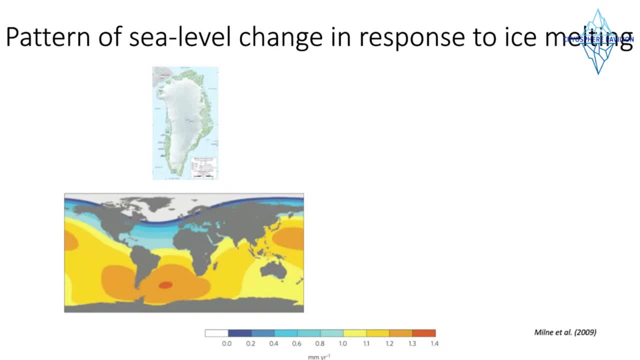 And this is basically showing: if one melts one millimeter- one melts Greenland ice sheet to raise sea level by one millimeters per year, then the regions in gray will experience sea level fall and regions in blue will experience sea level fall, rise but smaller than the value of globally global mean value. and red and orange yellow. 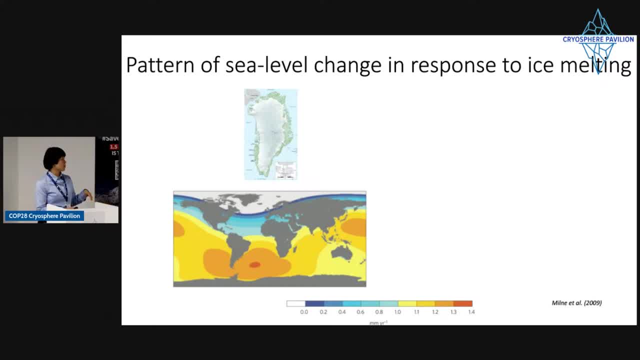 orange red regions are going to experience sea level rise greater than globally mean global mean average value. and this is what sea level pattern would look like when one melts antarctic ice sheet to raise sea level by one millimeters per year. um west antarctic ice sheet to be more. 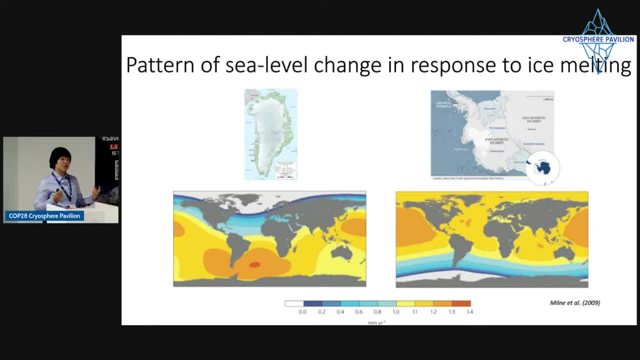 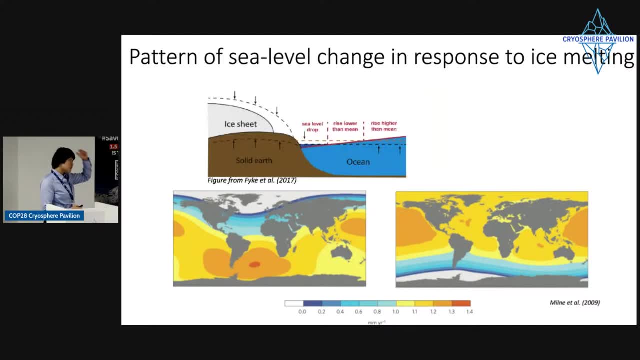 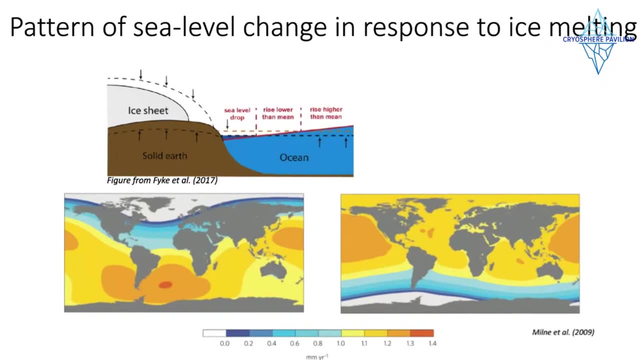 precise, so we can really see that the sea level change respond in response to ice sheet melting has its own fingerprint, and the physics of that is the following: first of all, when ice sheet melts, there is this um instantaneous and slow deformation of the solid earth. so more like 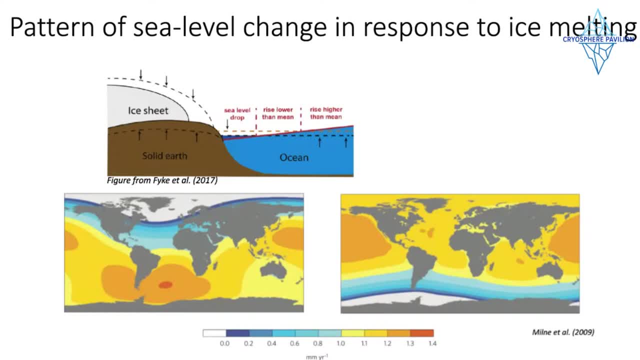 uplifting solid earth in response to unloading of the ice and ice sheet is a giant ice sheet and it's a giant ice sheet. and it's a giant ice sheet and it's a giant ice sheet, giant mass. so when it's there, it attracts ocean water close to its body, but as it melts away. 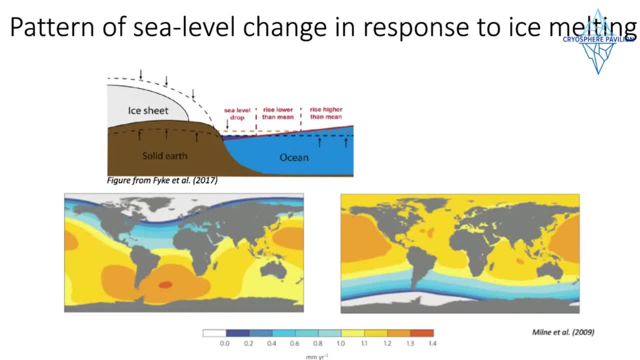 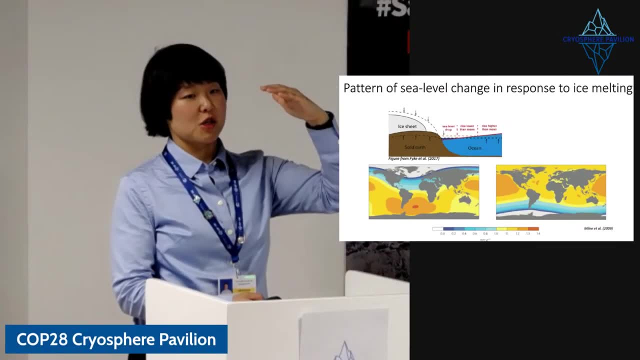 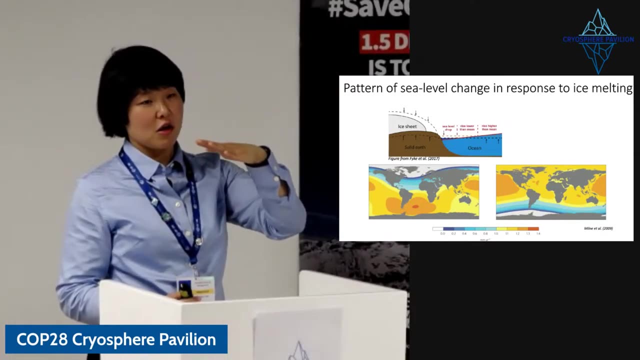 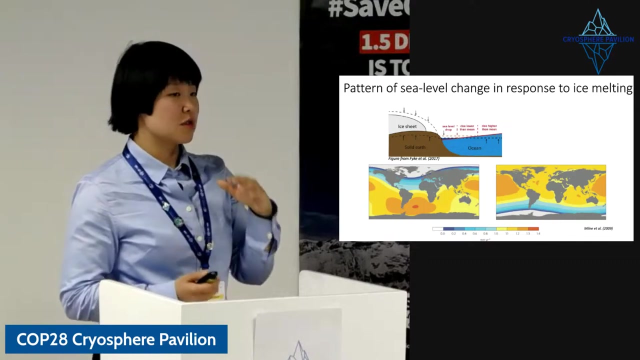 the ocean water near ice will migrate away from the retreating ice sheet. so the combination of this gravitational weakening, of gravitational attraction of ice into ice, thus um causing sea surface height fall, combination of that effect and also the uplift of the earth together causes the local sea level fall near the retreating region. and that's what's. 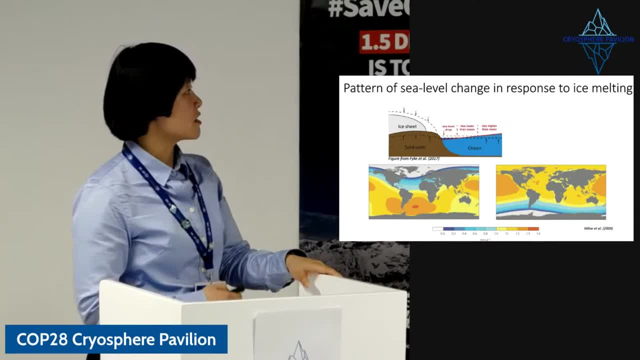 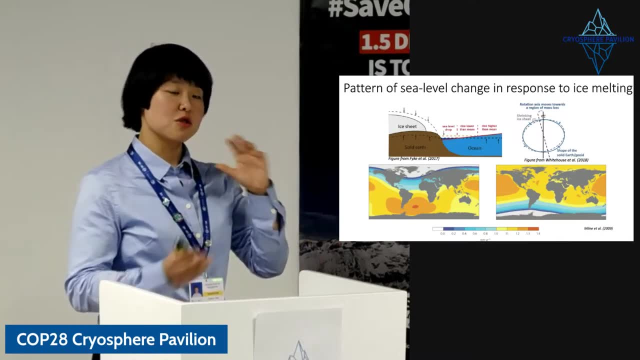 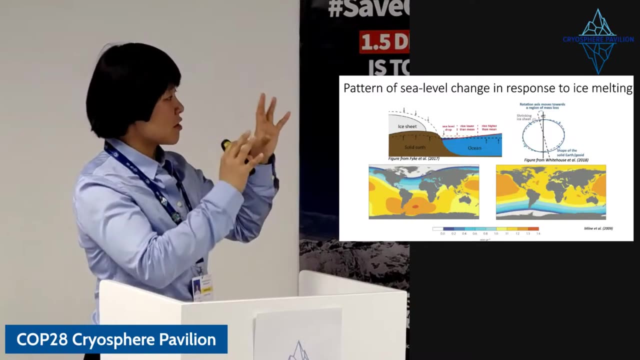 happening in these gray regions, um in the bottom plots. at the same time, um ice sheet retreated. the retreating ice sheet in the polar region causes shifting in the rotation vector vector of the earth, so it also then imprints this quadrature, um quadratic or quadrature pattern, on the globe. 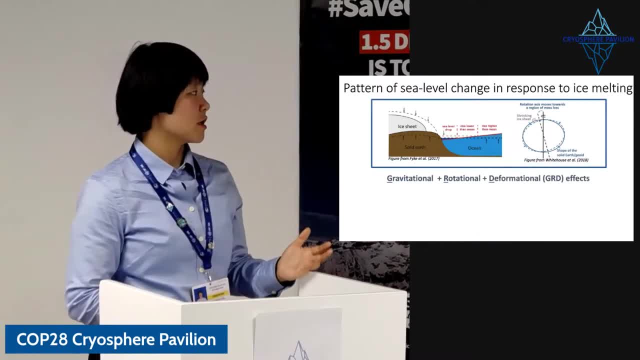 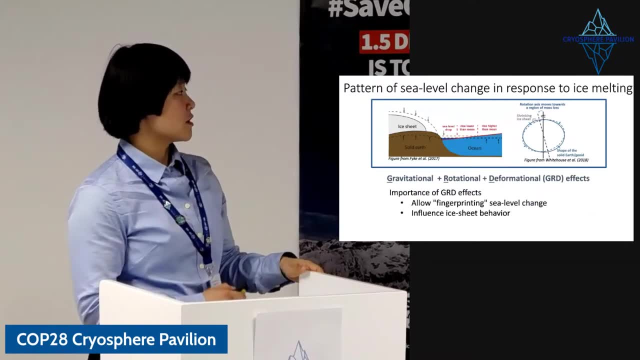 so all these effects together are all these effects together are called grd effects. gravitational, called grd effects. gravitational, rotational and deformational effects. rotational and deformational effects and the importance of grd effects is that, and the importance of grd effects is that, and the importance of grd effects is that it allows us, when we understand this, 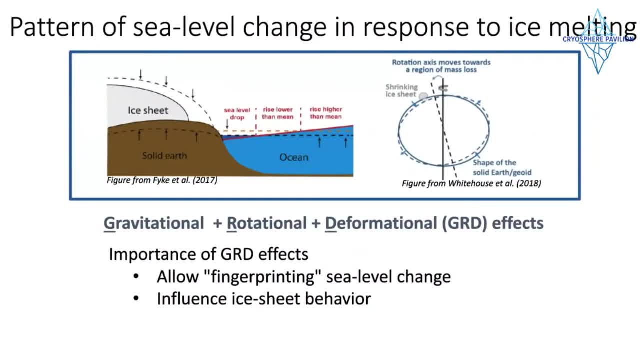 it allows us when we understand this. it allows us when we understand this: processes, processes, processes. it allows us to fingerprint sea level. it allows us to fingerprint sea level. it allows us to fingerprint sea level, change associated with ice melting, change associated with ice melting, change associated with ice melting and also this grd effects in turn. 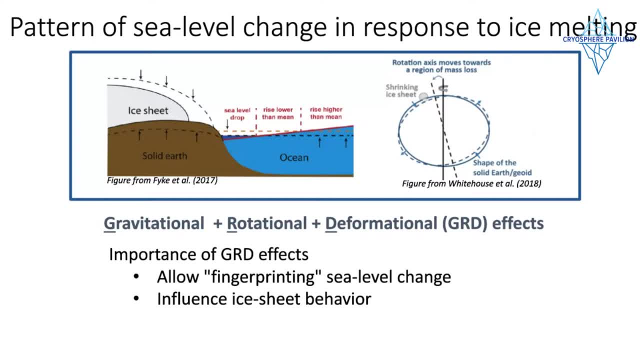 and also this grd effects in turn, and also this grd effects in turn influence the ice sheet behavior, influence the ice sheet behavior, influence the ice sheet behavior. so this fit. there's this feedback, so this fit. there's this feedback, so this fit. there's this feedback between ice sheet and grd effects. so ice. 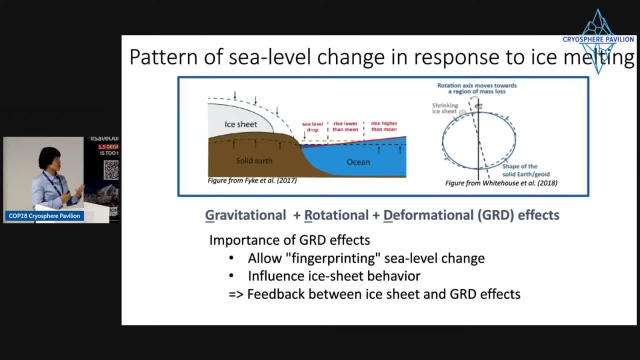 between ice sheet and grd effects. so ice. between ice sheet and grd effects. so ice sheet changes in response to climate sheet changes. in response to climate sheet changes. in response to climate change and grd effects: response in change and grd effects. response in change and grd effects. response in response to ice sheet. 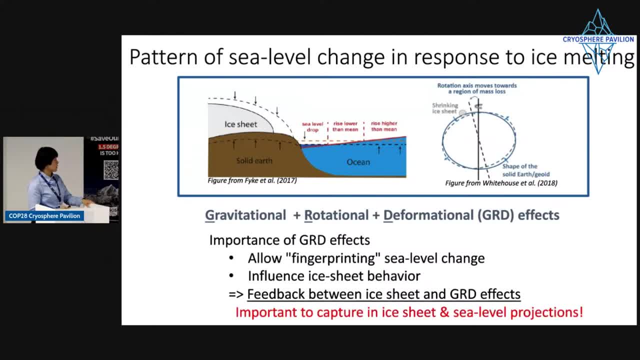 response to ice sheet. response to ice sheet in turn affects the ice sheet dynamics. in turn affects the ice sheet dynamics. in turn affects the ice sheet dynamics. so this feedback is really important to, so this feedback is really important to, so this feedback is really important to capture in projecting both ice sheet and. 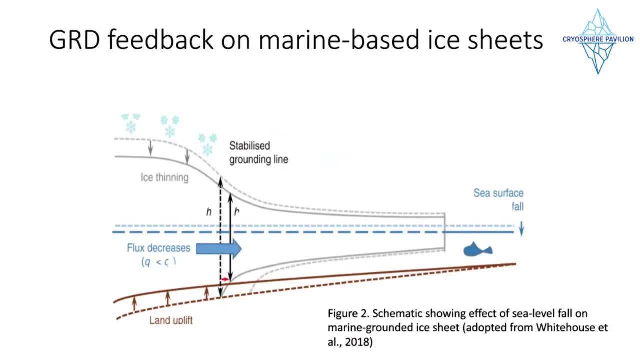 capture in projecting both ice sheet and capture in projecting both ice sheet and sea level, sea level: sea level. and so this grd effect is especially, and so this grd effect is especially, and so this grd effect is especially important to capture in ice sheet, important to capture in ice sheet. 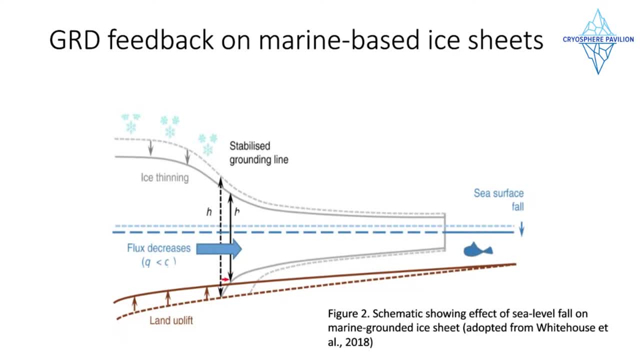 important to capture in ice sheet region. so that means that if ice sheet region, so that means that if ice sheet region, so that means that if ice sheet is, is is sitting below the ocean, um sitting below the ocean, um sitting below the ocean, um ice sheet is pretty unstable. i will. 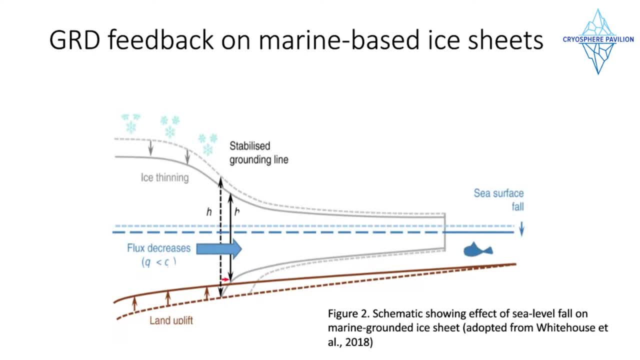 ice sheet is pretty unstable. i will: ice sheet is pretty unstable. i will especially um, especially um, especially um. well, i guess i have to first, i'll first. well, i guess i have to first, i'll first. well, i guess i have to first, i'll first introduce. 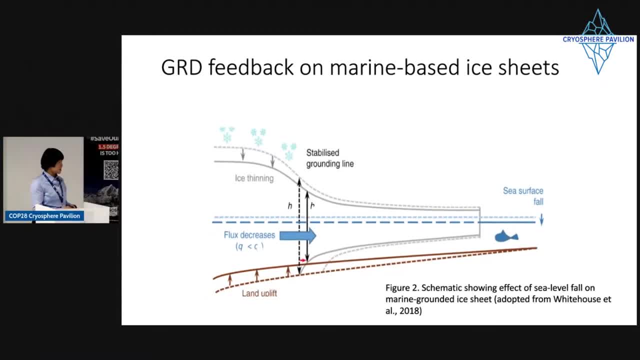 introduce, introduce the dynamics of it or physics of it. so the dynamics of it or physics of it. so the dynamics of it or physics of it. so when an ice sheet is sitting, when an ice sheet is sitting, when an ice sheet is sitting on a bed, especially when the bed slope, 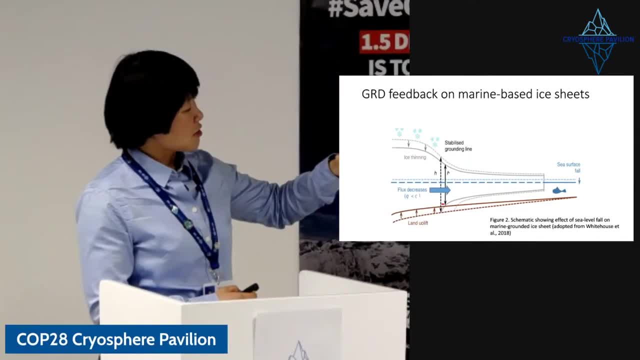 on a bed, especially when the bed slope on a bed, especially when the bed slope, that is going. the depth of the bed is that is going. the depth of the bed is that is going. the depth of the bed is increasing, increasing, increasing, going inland and going inland and 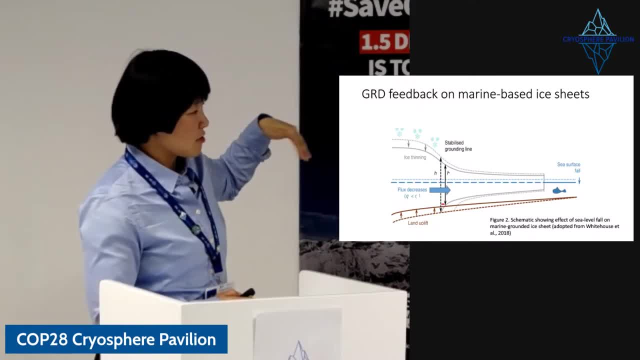 going inland and the ice sheet loses mass across its. the ice sheet loses mass across its. the ice sheet loses mass across its grounding line, which is where the ice grounding line, which is where the ice grounding line, which is where the ice sheet starts to float into sheet starts to float into. 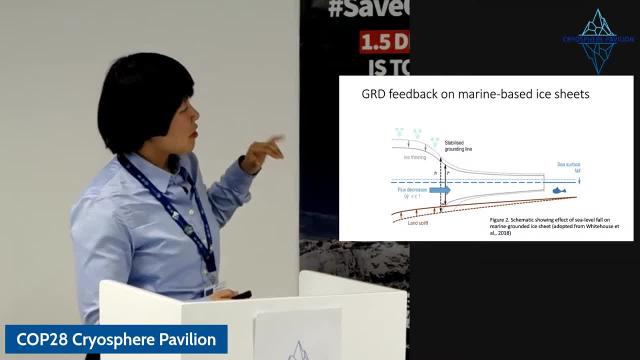 sheet starts to float into what um into the ocean, what um into the ocean, what um into the ocean. and so the thickness of the ice sheet, and so the thickness of the ice sheet, and so the thickness of the ice sheet at the grounding line is proportional to 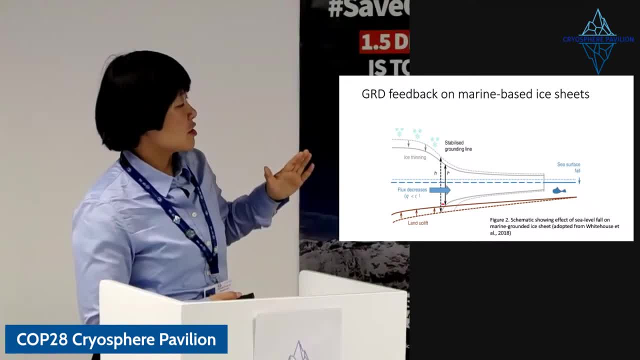 at the grounding line is proportional to: at the grounding line is proportional to the depth of the ocean there, the depth of the ocean there, the depth of the ocean there. and so, if the ice sheet is sitting on a, and so if the ice sheet is sitting on a, 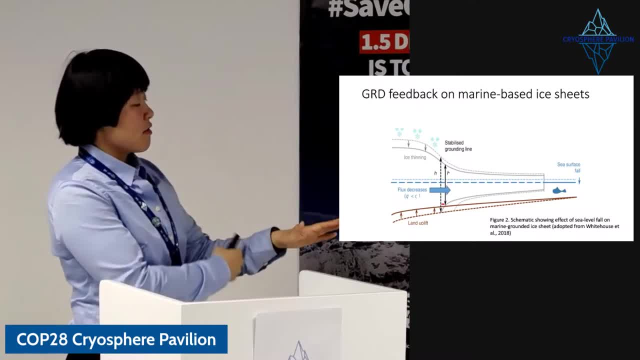 and so if the ice sheet is sitting on a bedrock that is going deeper and deeper bedrock that is going deeper and deeper bedrock that is going deeper and deeper inland, then that means that the ice inland, then that means that the ice inland, then that means that the ice sheet thickness. 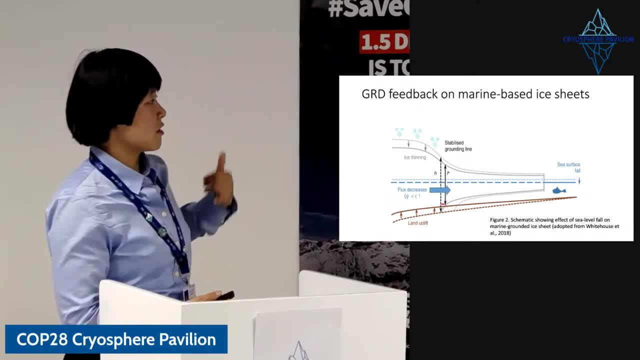 sheet thickness. sheet thickness at the grounding line. as the grounding at the grounding line, as the grounding at the grounding line as the grounding line retreats backward line, retreats backward line, retreats backward is also going to increase and therefore is also going to increase and therefore, 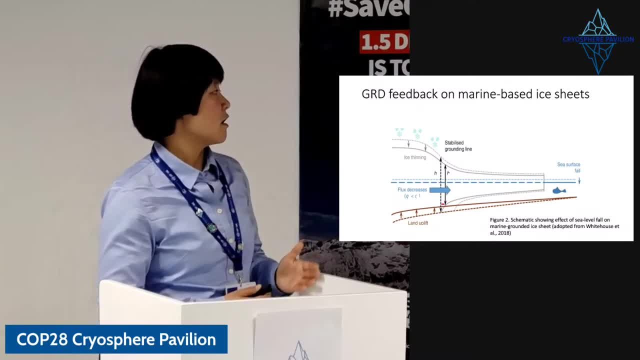 is also going to increase and therefore there is increase in flux of the ice. there is increase in flux of the ice, there is increase in flux of the ice across the grounding line and that across the grounding line, and that across the grounding line, and that is going to cause this feedback and 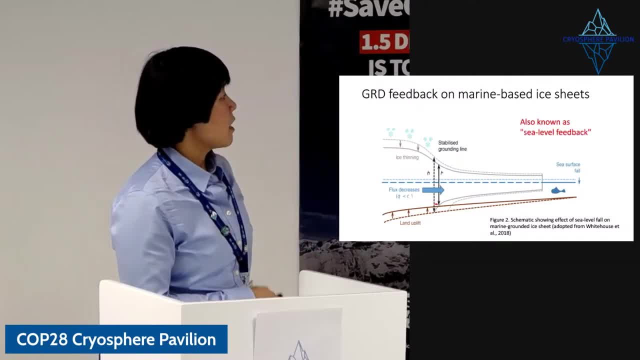 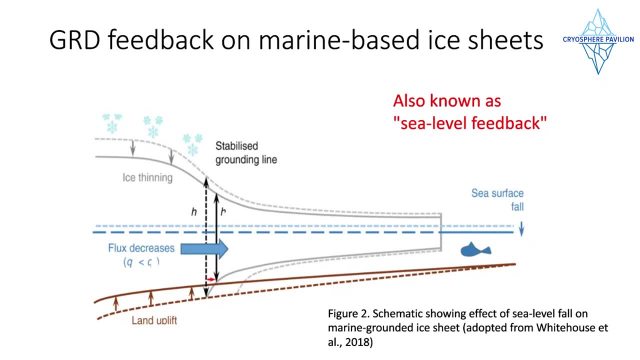 is going to cause this feedback and is going to cause this feedback and runaway effect of ice sheet. so when we incorporate the grd effects, so when we incorporate the grd effects, so when we incorporate the grd effects, which captures this uplift of the, which captures this uplift of the, 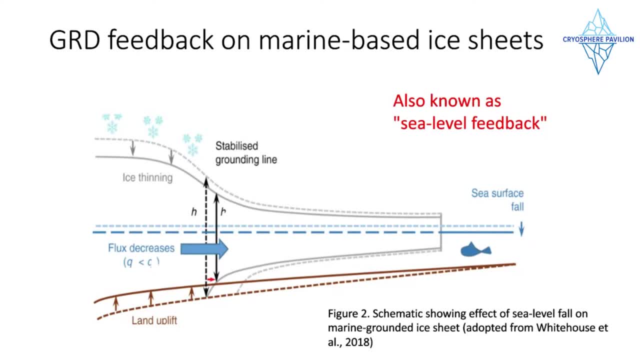 which captures this uplift of the solid earth and dropping of the sea solid earth and dropping of the sea solid earth and dropping of the sea surface height, causing local sea level surface height, causing local sea level surface height, causing local sea level fall, fall, fall then now what it used to be on the 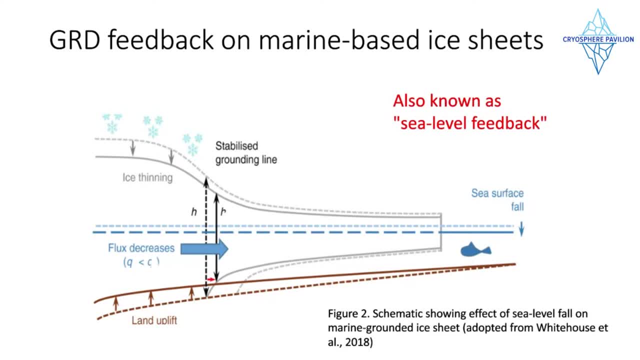 then now what it used to be on the, then now what it used to be on the retrograde slope, retrograde slope, retrograde slope. as the ice sheet loses as fast the. as the ice sheet loses as fast the. as the ice sheet loses as fast the, solid earth is bumping up and the sea. 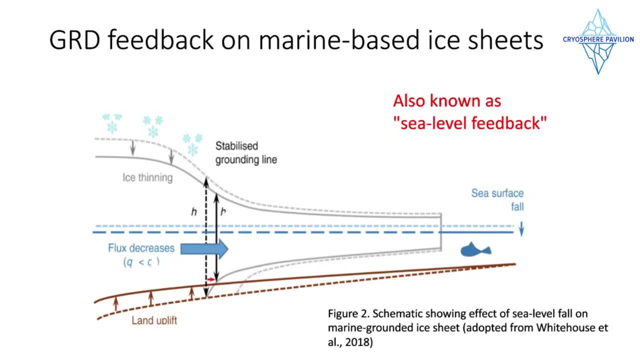 solid earth is bumping up and the sea solid earth is bumping up and the sea level is falling. level is falling. level is falling so that causes or that feeds back into, so that causes or that feeds back into, so that causes or that feeds back into the ice sheet. and 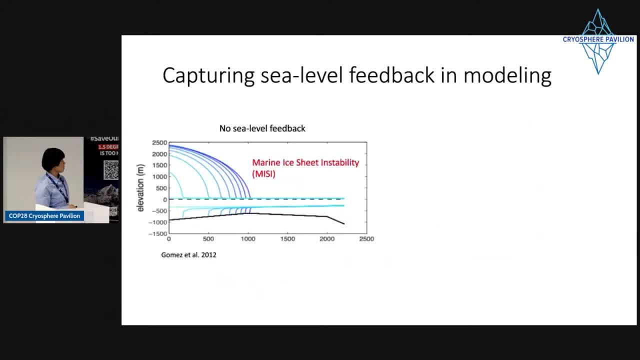 the ice sheet and the ice sheet and acts as a stabilizing factor. so this is a demonstration of using a. so this is a demonstration of using a. so this is a demonstration of using a simple model, simple model, simple model. and when there is no sea level feedback. 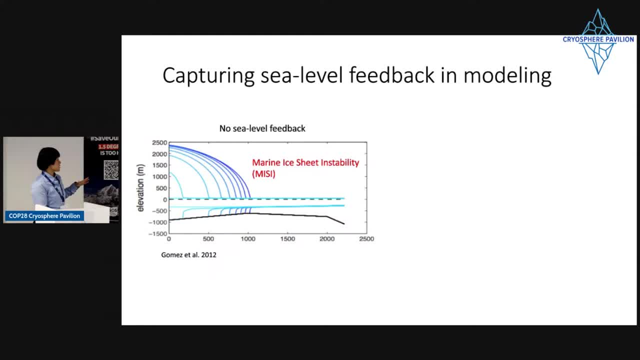 and when there is no sea level feedback and when there is no sea level feedback or grd feedback, or grd feedback or grd feedback on a marine-based ice sheet, on a on a marine-based ice sheet, on a on a marine-based ice sheet on a retrograde bed soap. if you just 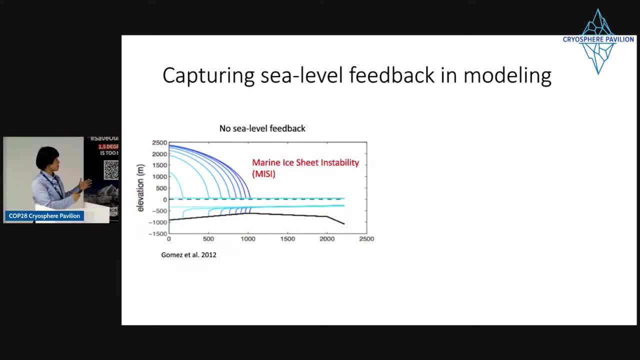 retrograde bed soap. if you just retrograde bed soap, if you just let the run ice sheet just retreat, or let the run ice sheet just retreat, or let the run ice sheet just retreat or evolve, then it's going to um experience evolve, then it's going to um experience. 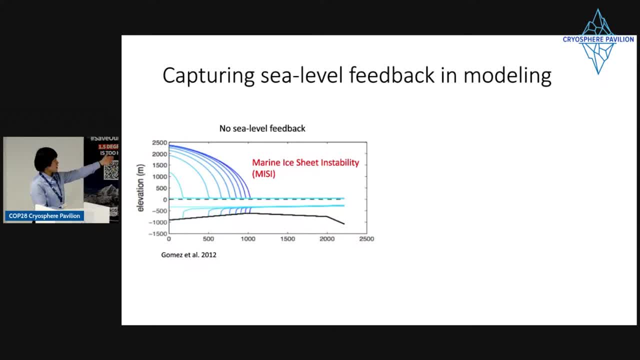 evolve, then it's going to um experience this runaway effect. so, going from this runaway effect, so going from this runaway effect, so going from very end, like the larger ice sheet in very end, like the larger ice sheet in very end, like the larger ice sheet in the blue. 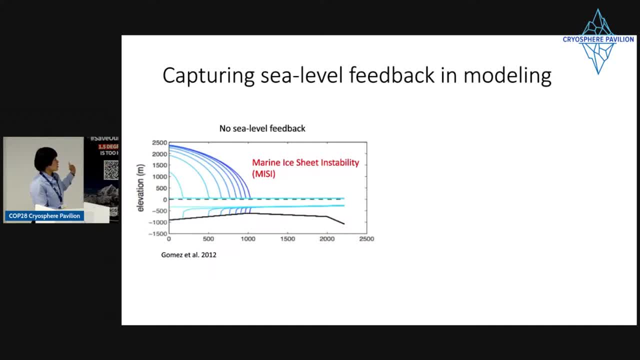 the blue, the blue, and then going all the way down to the, and then going all the way down to the, and then going all the way down to the light blue color. light blue color, light blue color scheme. and so this is this ice sheet scheme, and so this is this ice sheet. 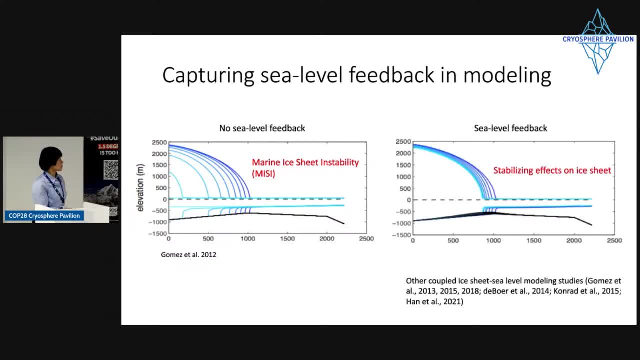 scheme. and so this is this: ice sheet experiences, what is called marine ice experiences, what is called marine ice experiences, what is called marine ice sheet instability, on the other hand, when, when one on the other hand, when, when one. on the other hand, when, when one incorporates sea level feedback. 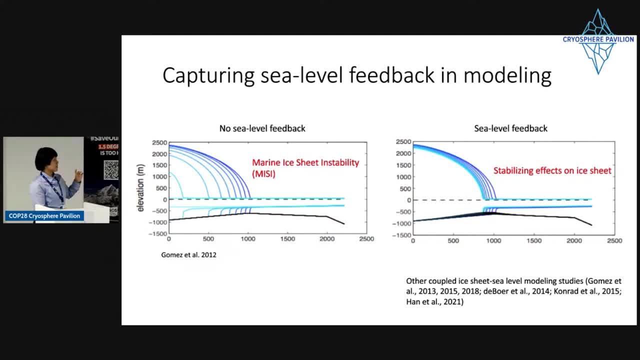 incorporates sea level feedback, incorporates sea level feedback, then the local sea level will fall, and then the local sea level will fall, and then the local sea level will fall and act as a stabilizing factor on onto. act as a stabilizing factor on onto, act as a stabilizing factor on onto this marine-based ice sheet, and you can. 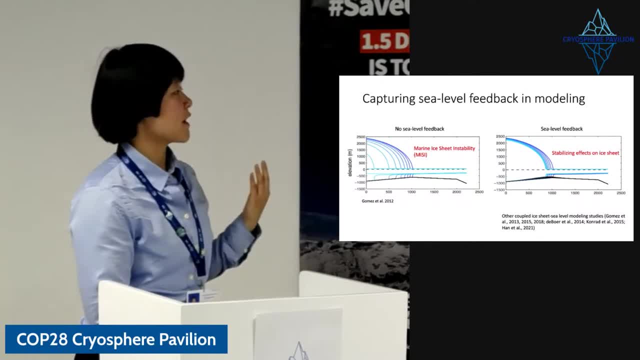 this marine-based ice sheet and you can this marine-based ice sheet and you can see that the ice sheet actually doesn't see that the ice sheet actually doesn't see that the ice sheet actually doesn't go through the runaway effect. go through the runaway effect, go through the runaway effect and this effect has been shown in the. 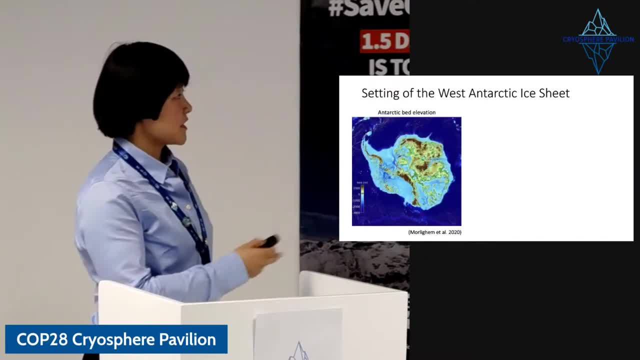 and this effect has been shown in the and this effect has been shown in the world. so this grd effects is really important. so this grd effects is really important. so this grd effects is really important to capture in, to capture in, to capture in places like east west antarctica, where you 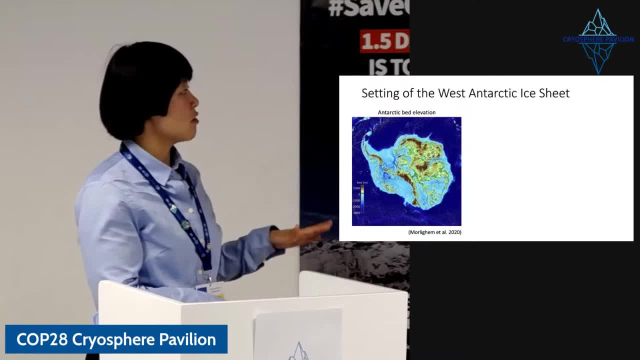 places like east west antarctica, where you places like east west antarctica, where you can see that the can see that the can see that the antarctic bed elevation goes below zero, antarctic bed elevation goes below zero. antarctic bed elevation goes below zero, which means that the bedrock is below. 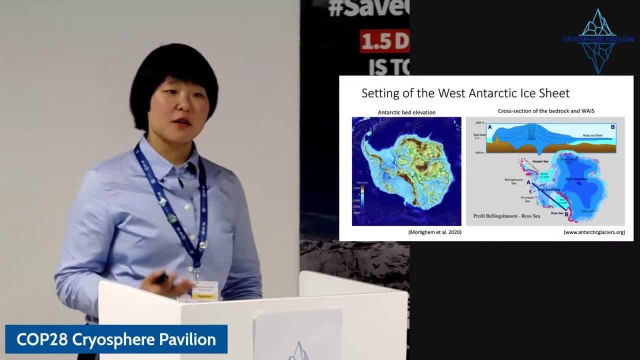 which means that the bedrock is below, which means that the bedrock is below sea level, sea level, sea level. and when you look at the cross section of, and when you look at the cross section of, and when you look at the cross section of the bedrock in, 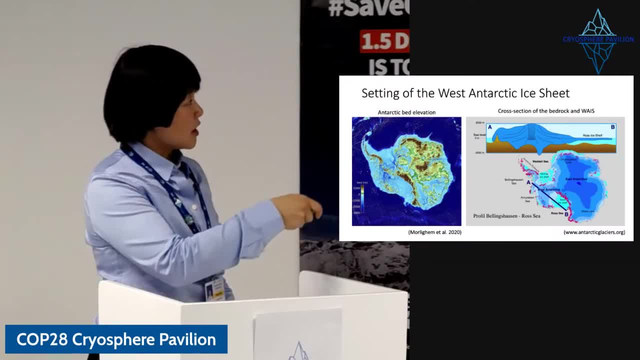 the bedrock in the bedrock in west antarctica. you can actually see that west antarctica. you can actually see that west antarctica. you can actually see that the, the, the ice sheet is marine based and then it sits. ice sheet is marine based and then it sits. 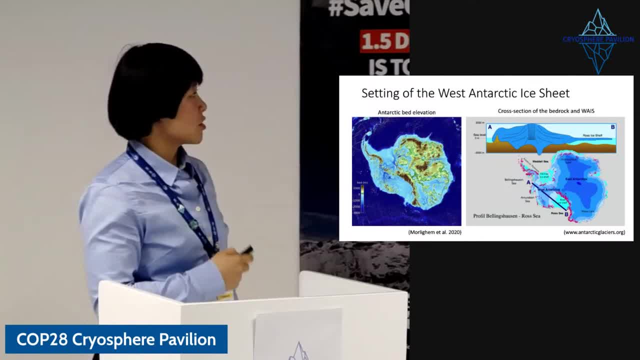 ice sheet is marine based and then it sits on on on that retrograde bedrock, so that retrograde bedrock, so that retrograde bedrock. so this grd effect is potentially very, this grd effect is potentially very, this grd effect is potentially very important, important, important to be captured in this setting, in the 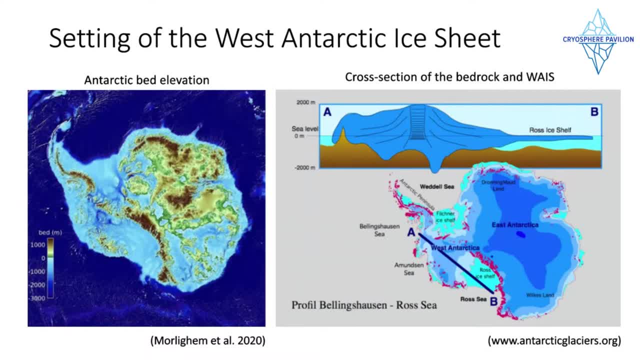 to be captured in this setting, in the to be captured in this setting in the west antarctic region, west antarctic region, west antarctic region, and also obviously um a couple of days, and also obviously um a couple of days and also obviously um a couple of days ago. 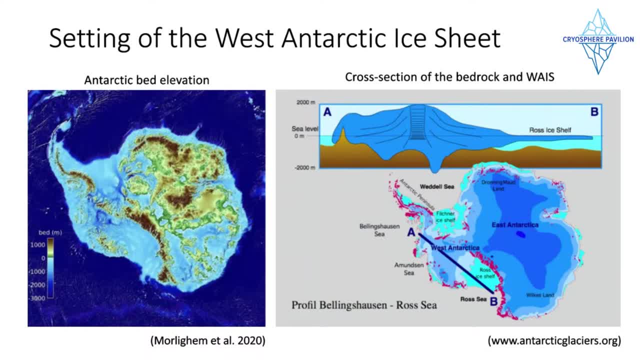 ago ago, chris stokes gave us a talk on uh focusing. chris stokes gave us a talk on uh focusing. chris stokes gave us a talk on uh focusing on eastern antarctica, on eastern antarctica, on eastern antarctica, in eastern tardy ice sheet and there are 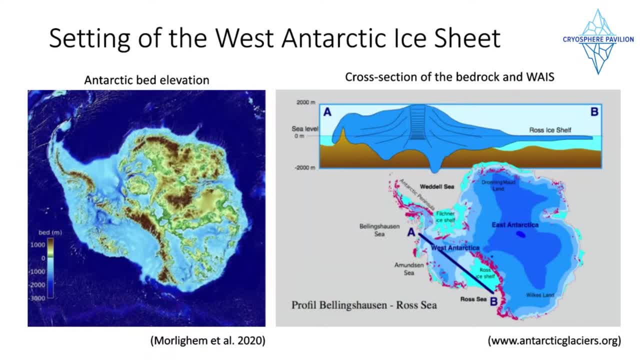 in eastern tardy ice sheet and there are in eastern tardy ice sheet and there are three marine based issues that are also three marine based issues that are also three marine based issues that are also behaving or situated in a pretty behaving or situated in a pretty. 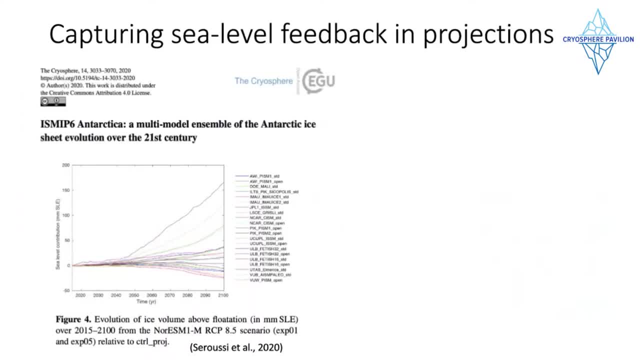 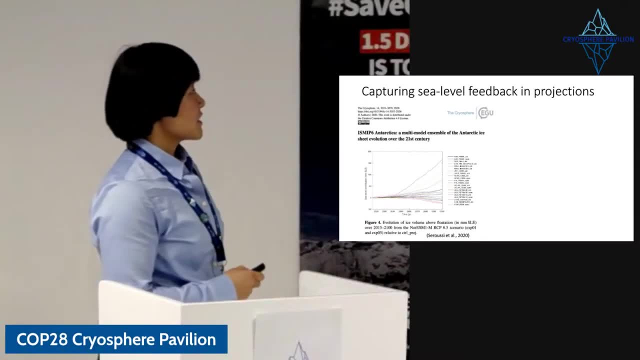 behaving or situated in a pretty similar setting as the west antarctic, similar setting as the west antarctic, similar setting as the west antarctic ice sheet here. so going into my topic of research, so going into my topic of research, so going into my topic of research, this 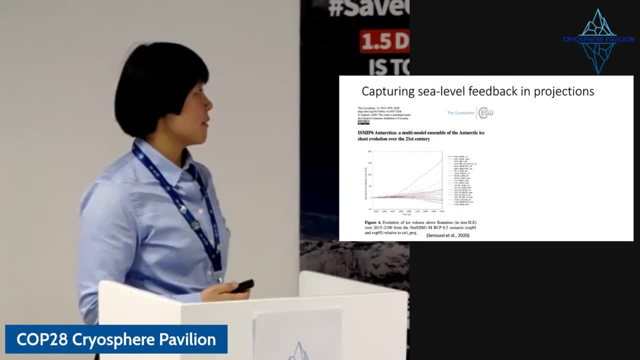 this. this grd effects or sea level feedback. grd effects or sea level feedback. grd effects or sea level feedback is important in, is important in. is important in. important for projecting ice sheet. important for projecting ice sheet. important for projecting ice sheet. contribution to sea level. contribution to sea level. 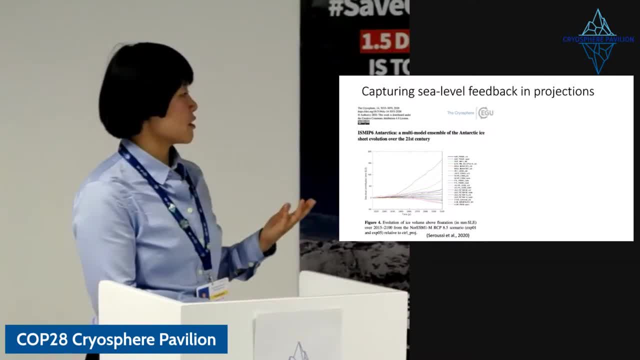 contribution to sea level, and there is this paper that was, and there is this paper that was, and there is this paper that was published in 2020 by sarah seattle, published in 2020 by sarah seattle, published in 2020 by sarah seattle, who did this amazing work of 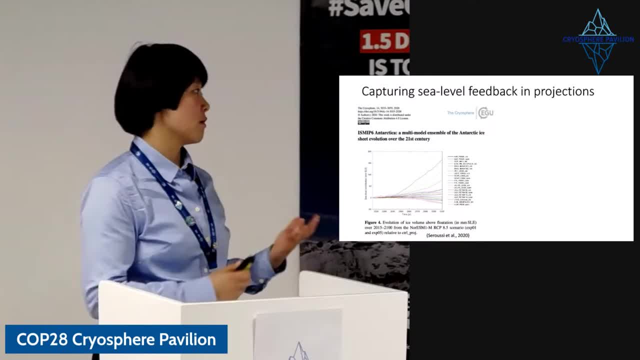 who did this amazing work of who did this amazing work of collaborating and combining all the collaborating and combining all the collaborating and combining all the projections from projections, from projections from ice sheet models across the world, and ice sheet models across the world and ice sheet models across the world, and provided the projections of sea level. 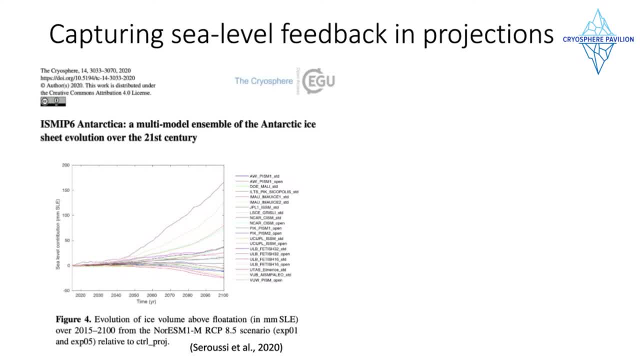 provided the projections of sea level. provided the projections of sea level in over the 21st century, in over the 21st century, in over the 21st century. designs are projections of sea level by designs are projections of sea level by designs are projections of sea level by all different ice sheet modeling groups. 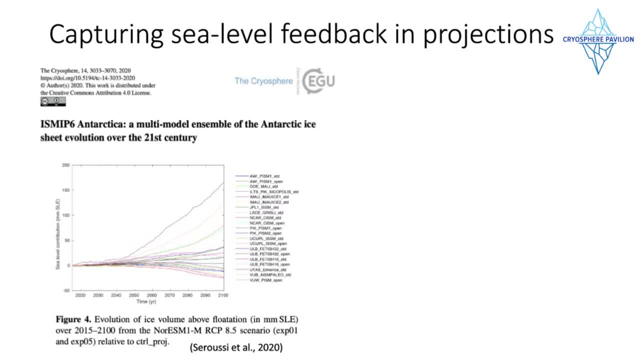 all different ice sheet modeling groups, all different ice sheet modeling groups across the world, across the world, across the world world. but in this plot world, but in this plot world, but in this plot, there are no grd effects. there are no. there are no grd effects, there are no. 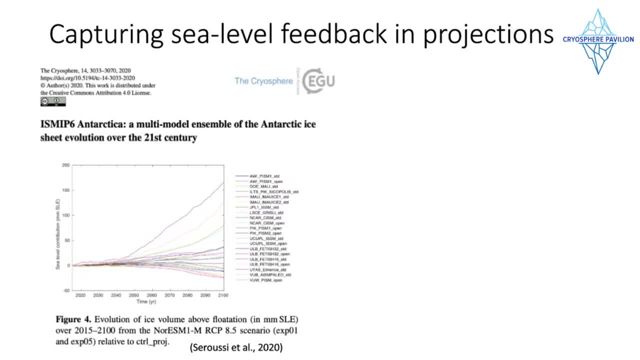 there are no grd effects. there are no ice sheet models. that ice sheet models, that ice sheet models, that that are who's capturing grd effects, that are who's capturing grd effects, that are who's capturing grd effects, and that is really not to blame. and that is really not to blame. 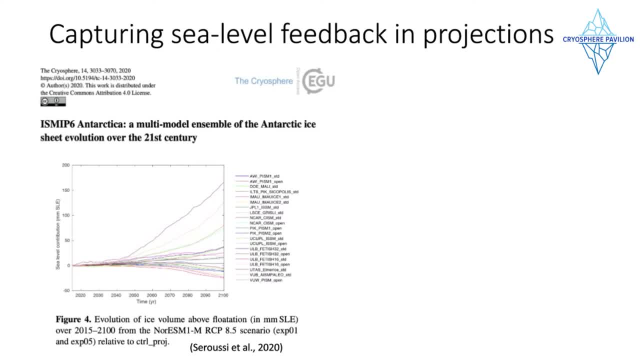 and that is really not to blame because um grd effects or what is also because um grd effects, or what is also because um grd effects, or what is also called, used to be called g, called, used to be called g, called, used to be called g, what is also known as gia effects in the 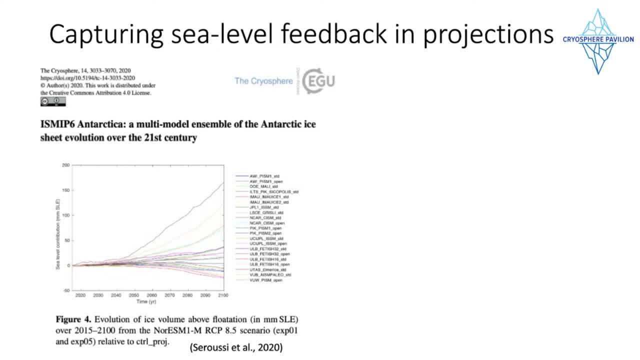 what is also known as gia effects in the, what is also known as gia effects in the paleo community- paleo community, paleo community- used to be known as really important, for used to be known as really important, for used to be known as really important for long time scale. 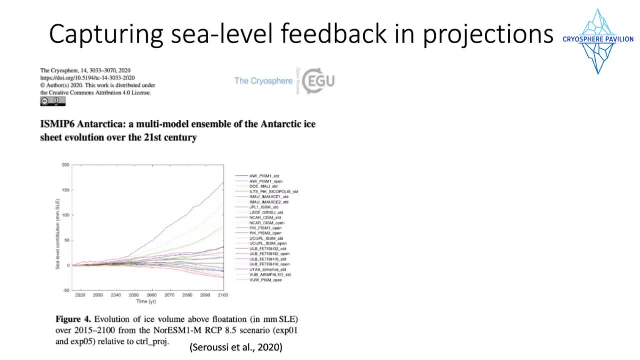 long time scale. long time scale ice dynamics, but not really for the ice dynamics, but not really for the ice dynamics, but not really for the future. like short-term future. like short-term future. like short-term, decadal or even centennial time scale. decadal or even centennial time scale. 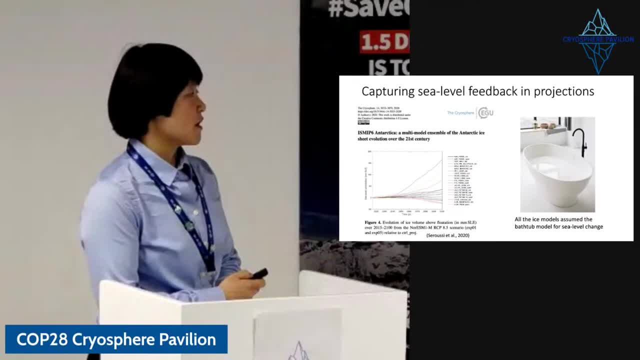 decadal or even centennial time scale, projections, projections, projections. so the grd effects have not been really so. the grd effects have not been really so. the grd effects have not been really captured in this future ice sheet. captured in this future ice sheet captured in this future ice sheet modeling community. 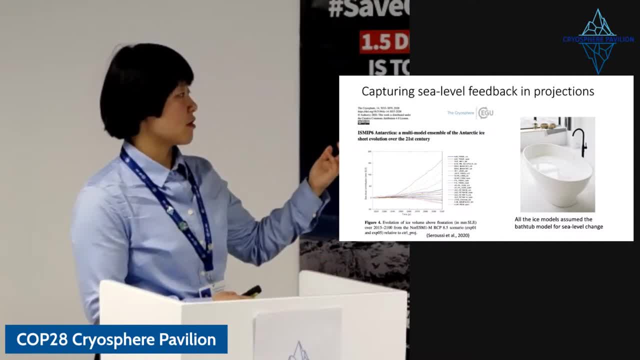 modeling community. modeling community worked, and so these ice sheet models worked, and so these ice sheet models worked, and so these ice sheet models either assume that the sea level change, either assume that the sea level change, either assume that the sea level change is globally uniform, is globally uniform. 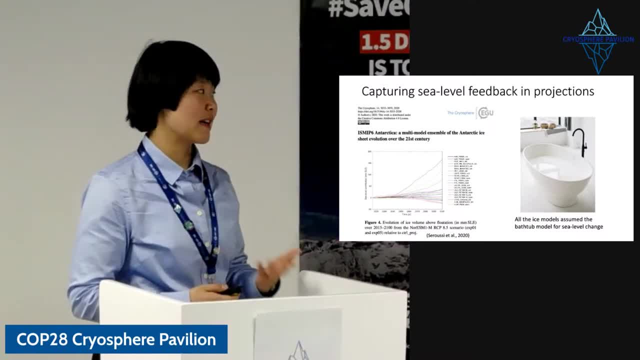 is globally uniform, or they just don't have sea level as a, or they just don't have sea level as a, or they just don't have sea level as a component at all. so here i'm working at los alamos. so here i'm working at los alamos. 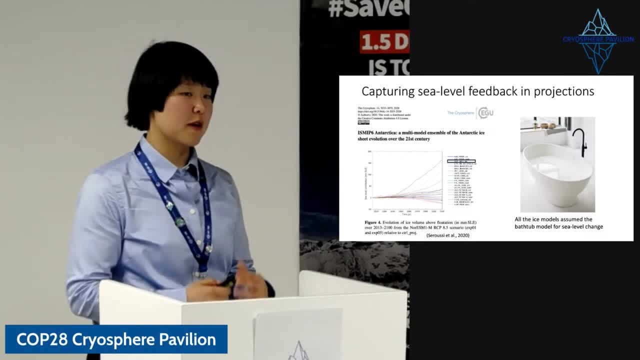 so here i'm working at los alamos national laboratory. i'm using national laboratory, i'm using national laboratory, i'm using us department of energy ice sheet model. us department of energy ice sheet model. us department of energy ice sheet model. component of the earth system model. 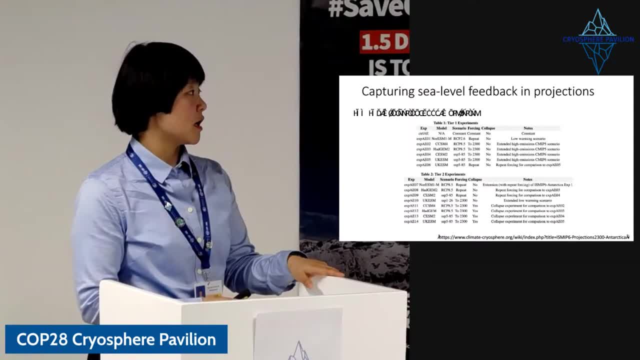 component of the earth system- model. component of the earth system- model molly. and so i've taken this model molly, and so i've taken this model molly, and so i've taken this model and i've um coupled or. and i've um coupled or. 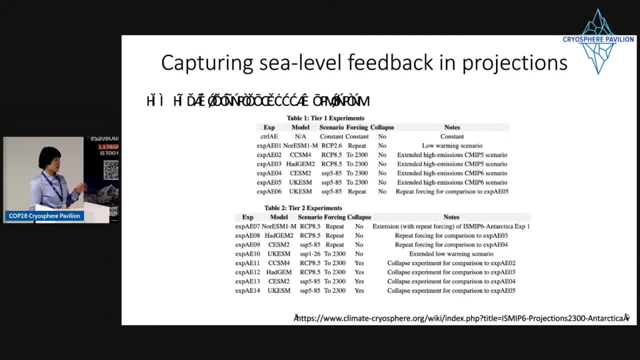 and i've um coupled or another in an easier term. i've made another in an easier term. i've made another in an easier term. i've made the ice sheet to be able to capture the, the ice sheet to be able to capture the, the ice sheet to be able to capture the grd effects. 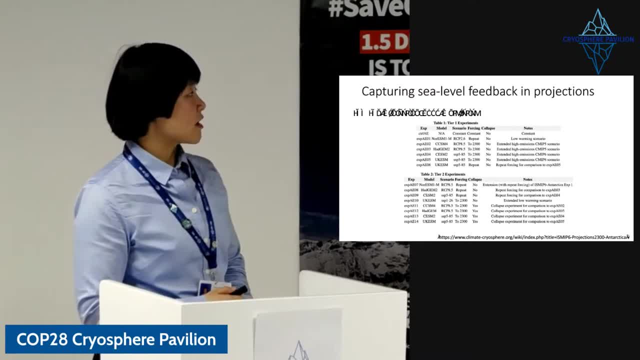 grd effects. grd effects and, and, and. ran through a variety of scenarios of, ran through a variety of scenarios of, ran through a variety of scenarios of ismip6, and i don't know why this text, ismip6, and i don't know why this text. 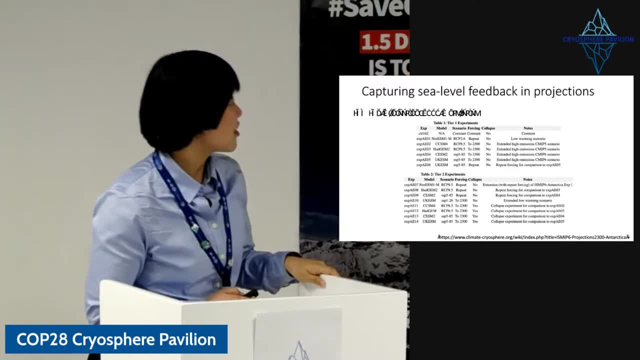 ismip6 and i don't know why this text keeps coming up. it doesn't show up on my keeps coming up. it doesn't show up on my keeps coming up. it doesn't show up on my slides where i think it's slides where i think it's. 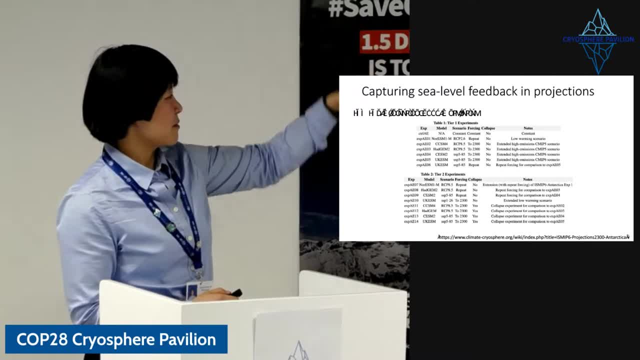 slides where i think it's yes, so yes, so yes. so ignore the text at the um in the middle. ignore the text at the um in the middle. ignore the text at the um in the middle. um is with six. um is with six. um is with six. published or. 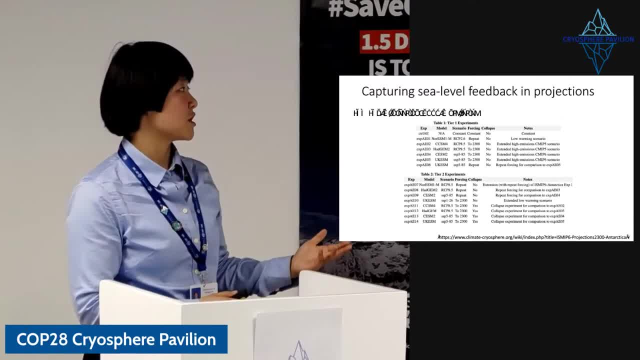 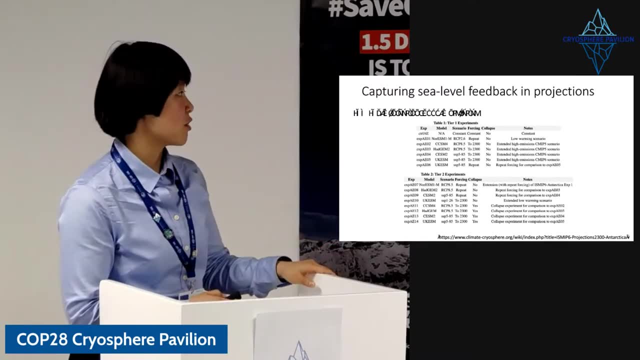 published or published or announced a new protocol in which the announced a new protocol, in which the announced a new protocol in which the climate forcing, climate forcing, climate forcing are extended up to 2300, are extended up to 2300, are extended up to 2300, as opposed to 21st 2100. 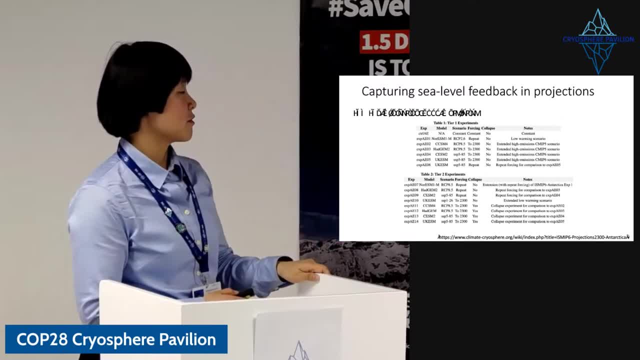 as opposed to 21st 2100, as opposed to 21st 2100. so these are all different type of, so these are all different type of. so these are all different type of experiments, but i'm focusing only on few experiments, but i'm focusing only on few. 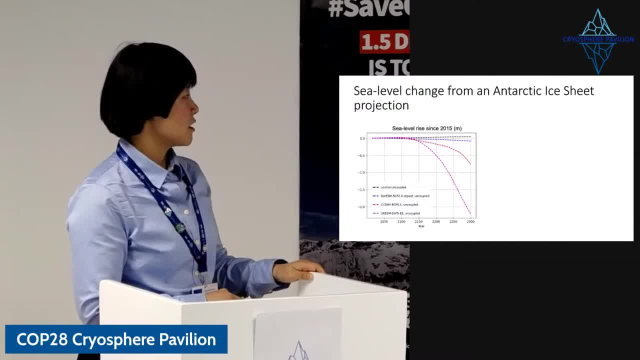 experiments, but i'm focusing only on few um, um, um. so i've taken, so i've taken, so i've taken some high-end and low-end forcing, some high-end and low-end forcing, some high-end and low-end forcing scenarios and apply to scenarios and apply to 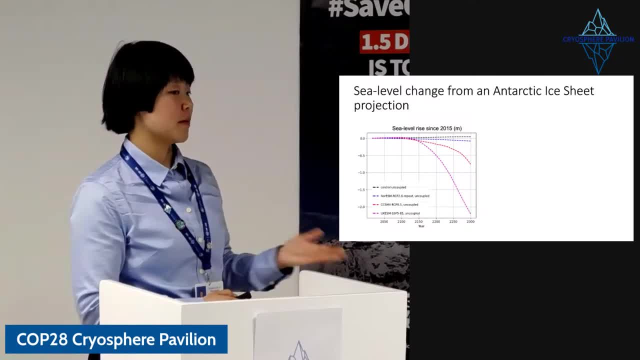 scenarios and apply to the molly ice sheet model and also the the molly ice sheet model and also the the molly ice sheet model, and also the coupled molly and sea level model- coupled molly and sea level model- coupled molly and sea level model, and so it is showing the sea level. 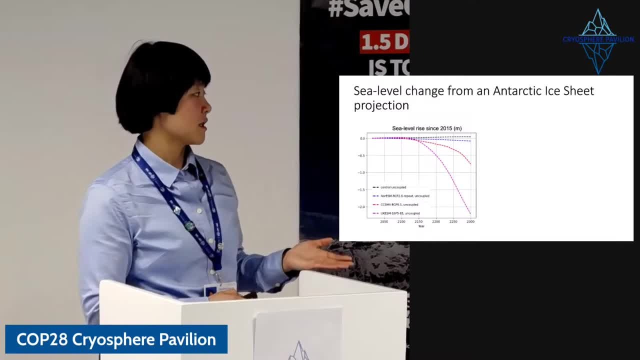 and so it is showing the sea level, and so it is showing the sea level projection of by molly through the next projection of by molly, through the next projection of by molly through the next 280 years, 280 years, 280 years. the blue line is showing the control. 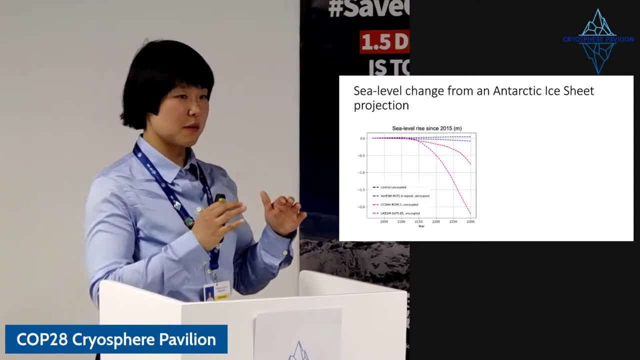 the blue line is showing the control. the blue line is showing the control: results control scenario. where results control scenario. where results control scenario. where the forcing climate forcing is just fixed: the forcing climate forcing is just fixed. the forcing climate forcing is just fixed to present day. to present day. 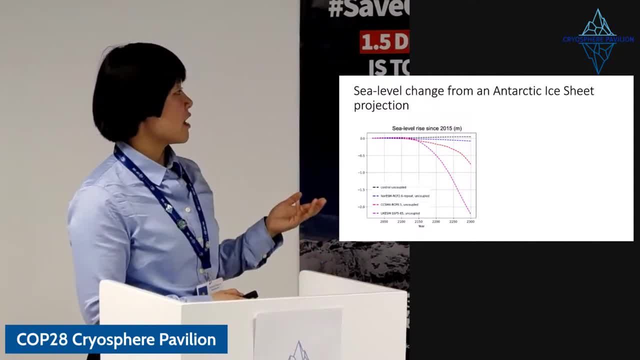 to present day and we're not really changing anything. and we're not really changing anything, and we're not really changing anything. and in the blue line is the low-end, and in the blue line is the low-end, and in the blue line is the low-end scenario where it's close to the paris. 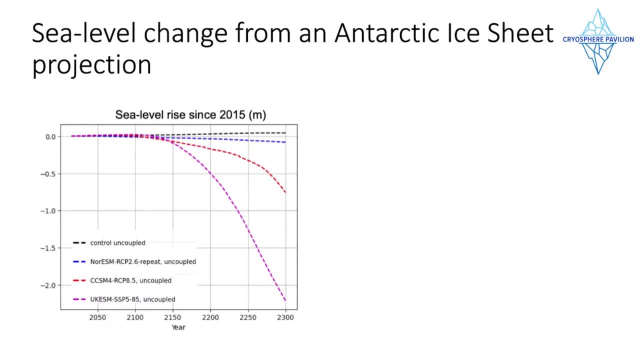 scenario where it's close to the paris scenario where it's close to the paris agreement goal, which is about one point agreement goal, which is about one point agreement goal, which is about one point, which is 1.5 degrees scenario, which is 1.5 degrees scenario. 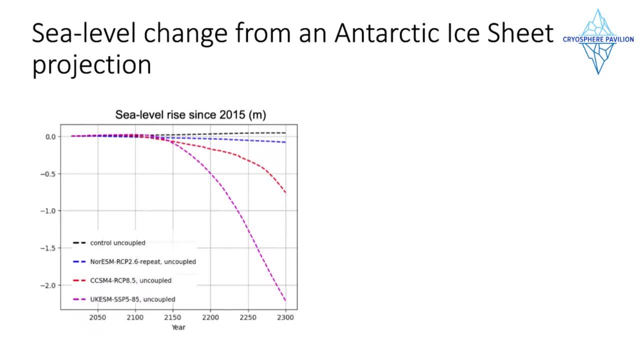 which is 1.5 degrees. scenario: warming and then the red line is warming, and then the red line is warming and then the red line is a little bit higher end climate, a little bit higher end climate, a little bit higher end climate, temperature temperature, temperature rise of about three degrees or four. 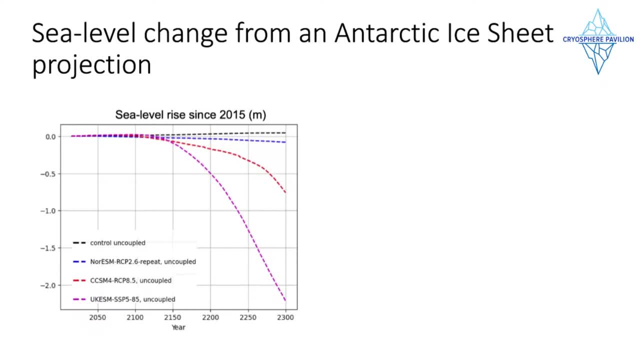 rise of about three degrees or four. rise of about three degrees or four degrees and same degrees and same degrees, and same for the purple line the bottom, but using for the purple line the bottom, but using for the purple line the bottom, but using different, different, different climate model. 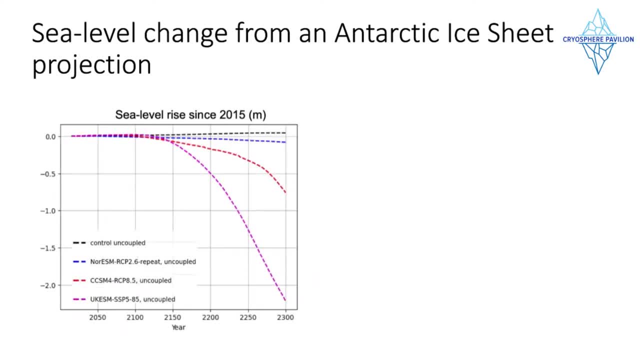 climate model, climate model. so the dash line here is showing so. the dash line here is showing so. the dash line here is showing the projection of ice sheet model. when the projection of ice sheet model, when the projection of ice sheet model, when it doesn't capture, it doesn't capture. 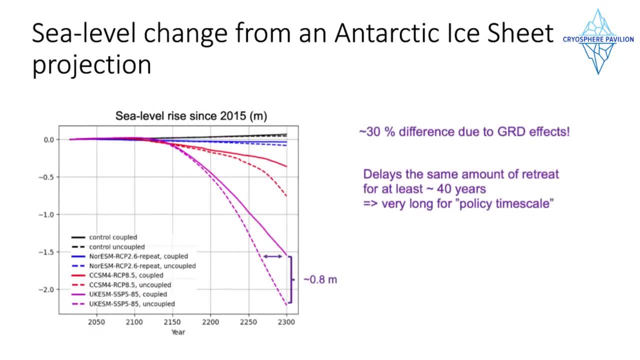 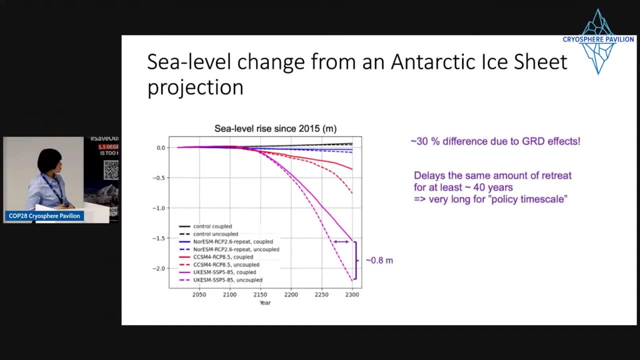 it doesn't capture grd effects and the solid lines, grd effects and the solid lines, grd effects and the solid lines. here now are showing the results of the here now are showing the results of the. here now are showing the results of the model, that model, that model that captures grd effects, and how to see this. 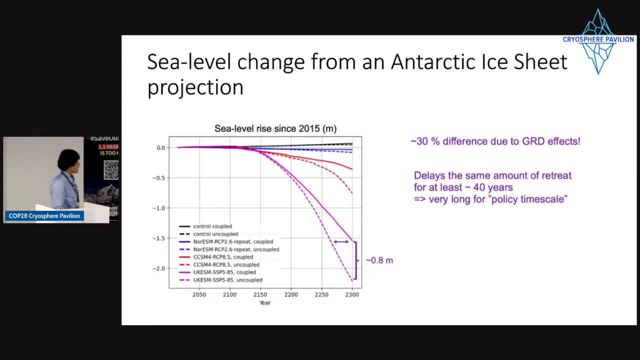 captures grd effects and how to see this. captures grd effects and how to see this. how to interpret this results? is you can? how to interpret this results? is you can? how to interpret this results? is you can see that the lines see that? the lines see that the lines are a little bit higher when the solid 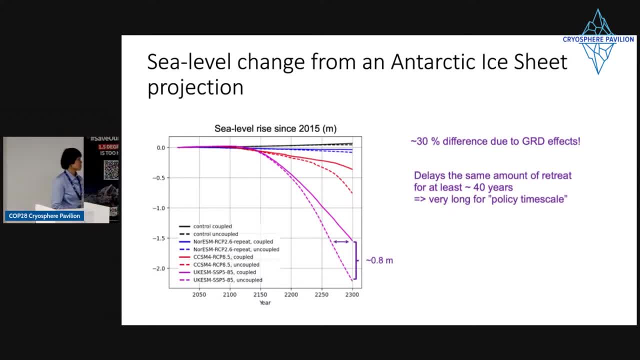 are a little bit higher when the solid are a little bit higher. when the solid lines are sitting higher, lines are sitting higher in when, when we're capturing grd effects in when, when we're capturing grd effects in when, when we're capturing grd effects, and that means that the ice sheet is 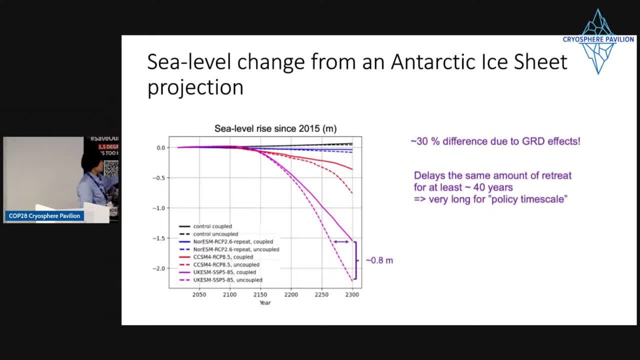 and that means that the ice sheet is, and that means that the ice sheet is melting less, melting less, melting less. and so the y-axis is sea level rise, and so the y-axis is sea level rise, and so the y-axis is sea level rise in liters. 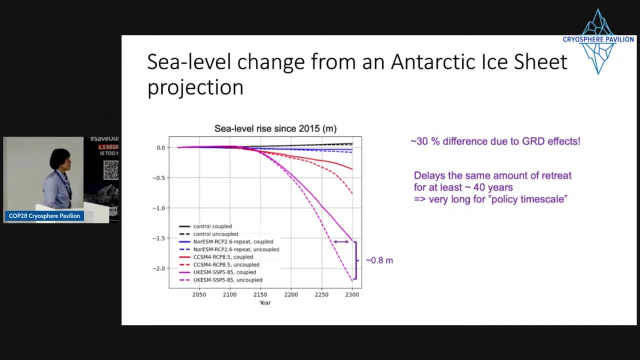 in liters. in liters, and x-axis is here and x-axis is here and x-axis is here until from 2015, until from 2015, until from 2015, up to 2300, up to 2300, up to 2300, and you can really see that this. 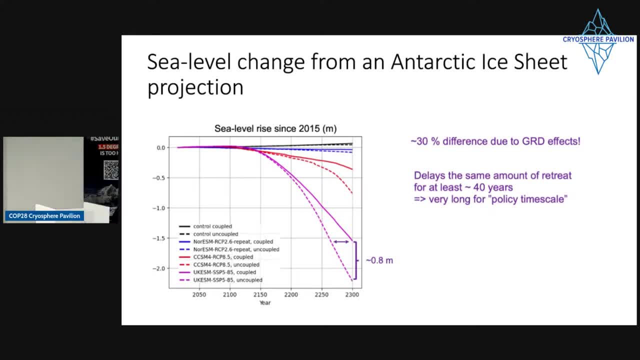 and you can really see that this and you can really see that this strength of the forcing in the very high strength of the forcing, in the very high strength of the forcing in the very high end forcing scenario, or strength of the end forcing scenario, or strength of the. 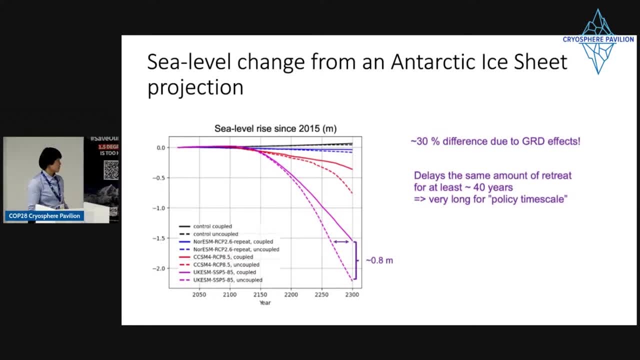 end forcing scenario or strength of the sea level feedback. sea level feedback- sea level feedback more precisely, is really strong. it more precisely, is really strong. it more precisely, is really strong. it maintains or retains more about maintains or retains. more about maintains or retains, more about retains- about 30 percent. 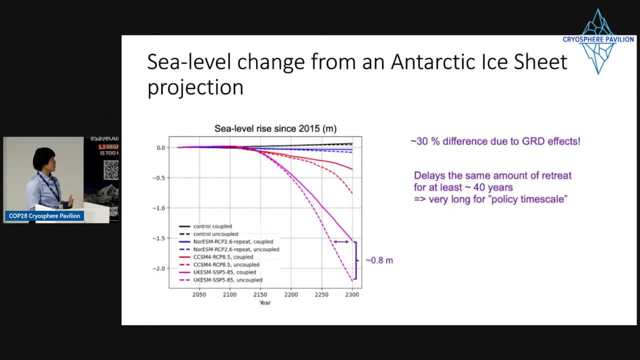 retains about 30 percent. retains about 30 percent. more ice when grd effects is captured and more ice when grd effects is captured, and more ice when grd effects is captured, and in number it's about 0.8 meters of. in number it's about 0.8 meters of. 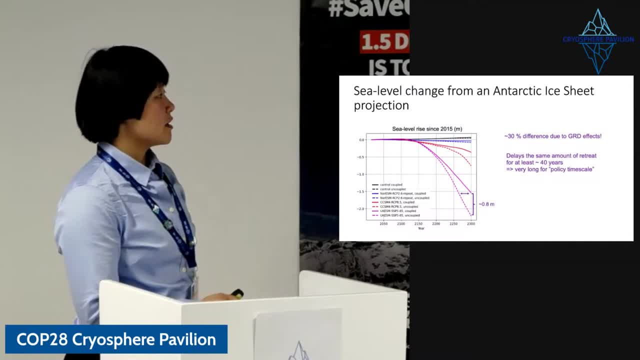 in number, it's about 0.8 meters of sea level equivalent ice volume, sea level equivalent ice volume, sea level equivalent ice volume, and and and so, so, so, and then if you go to, then, if you go to, then, if you go to lower and lower, enforcing then the amount. 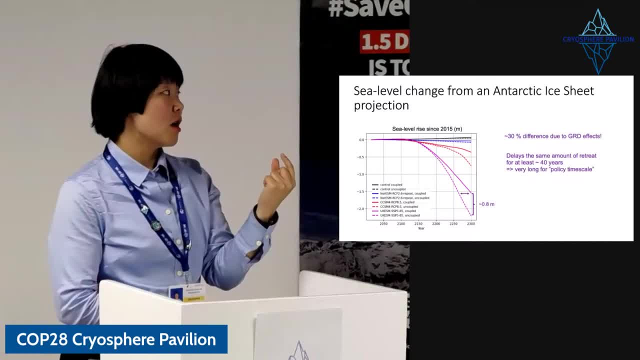 lower and lower, enforcing then the amount. lower and lower, enforcing then the amount of, or the strength of sea level feedback of, or the strength of sea level feedback of, or the strength of sea level feedback gets smaller, gets smaller, gets smaller. but actually the time it takes, but actually the time it takes. 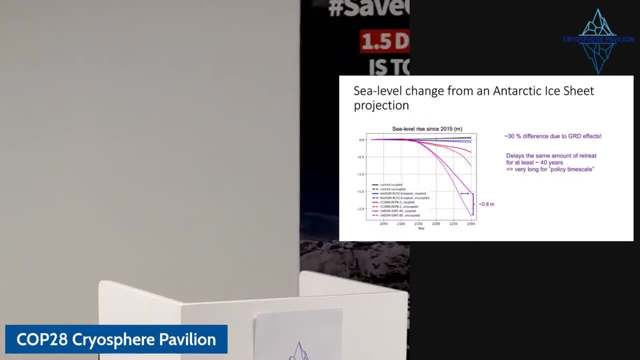 but actually the time it takes for ice sheet to melt, the same amount for ice sheet to melt. the same amount for ice sheet to melt. the same amount gets, gets, gets, it increases much, it increases much, it increases much, uh, much more, uh, much more, uh, much more so. 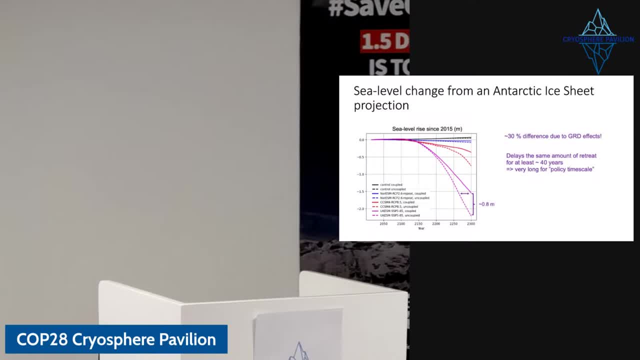 so, so, basically, basically, basically. in order to melt the same amount of, in order to melt the same amount of, in order to melt the same amount of ice in when we capture and share the ice in, when we capture and share the ice in, when we capture and share the effects there's about. 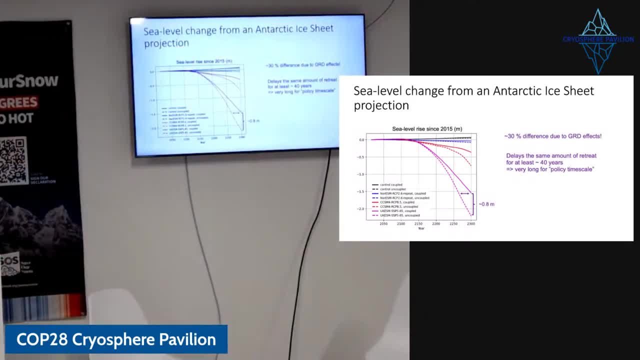 effects. there's about effects. there's about 40 years of delay, which is still pretty. 40 years of delay, which is still pretty. 40 years of delay, which is still pretty long for a policy time scale. long for a policy time scale, long for a policy time scale. um, but when you look at the blue lines, 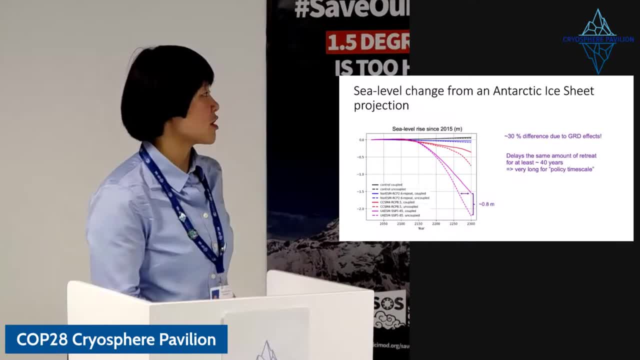 um, but when you look at the blue lines, um, but when you look at the blue lines and red lines, then the delay and red lines, then the delay and red lines, then the delay duration over delay time is gets duration over delay time is gets duration over delay time is gets longer. for example, for the red line, the 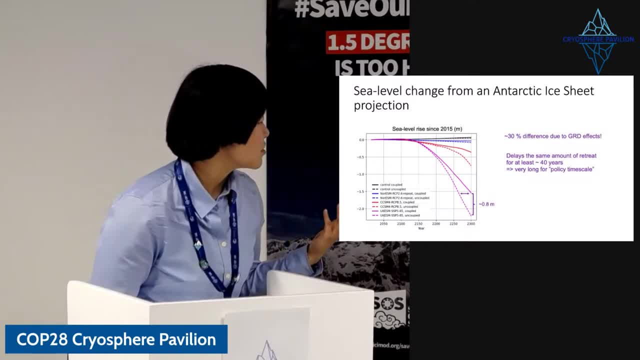 longer, for example, for the red line, the longer. for example, for the red line, the delay would be about 100 years. delay would be about 100 years. delay would be about 100 years for eight years, for eight years, for eight years and then for the blue line. it. 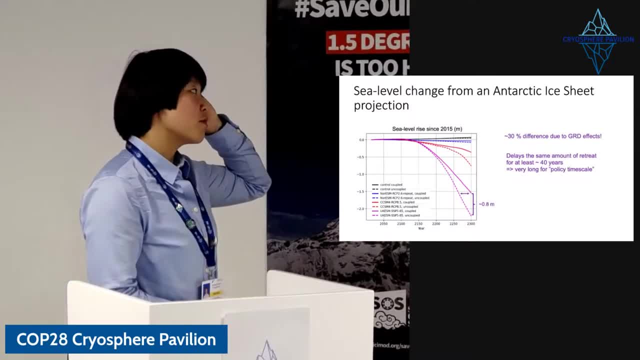 and then for the blue line it, and then for the blue line it: it's just yeah, it's just yeah, it's just yeah. gets way more, really longer. so it doesn't gets way more really longer. so it doesn't gets way more really longer. so it doesn't really. we don't really see the same. 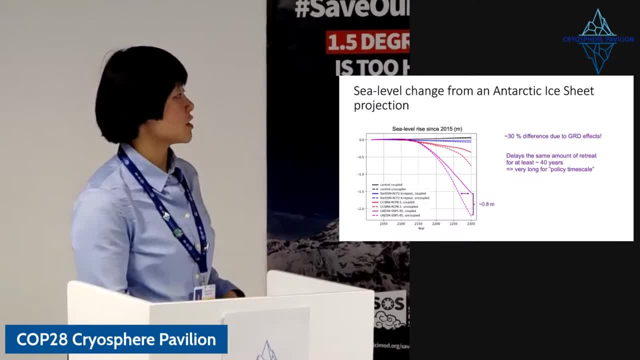 really we don't really see the same, really we don't really see the same amount of ice melting in this blue low amount of ice melting in this blue low amount of ice melting in this blue low enforcing scenario, enforcing scenario, enforcing scenario. so it really means that 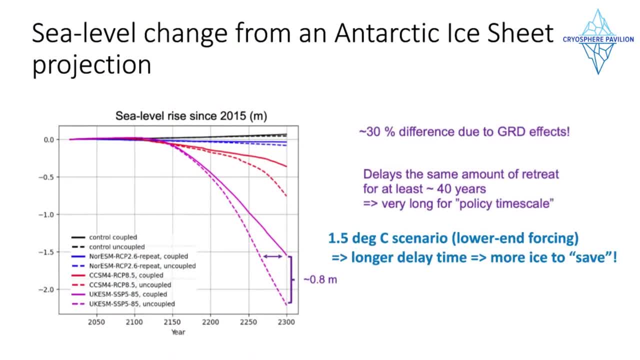 so it really means that. so it really means that in, in, in this 1.5 degree warming scenario, this 1.5 degree warming scenario, this 1.5 degree warming scenario, we can save a lot more ice. we can save a lot more ice. 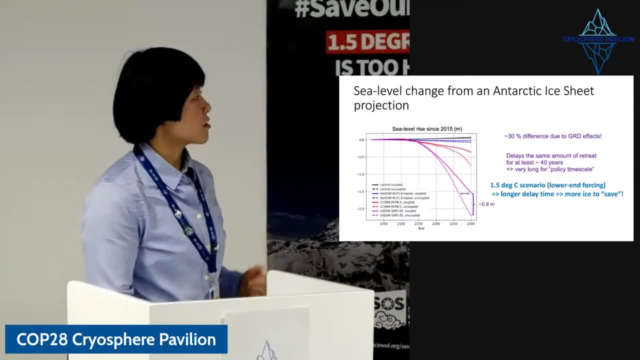 we can save a lot more ice. so there is it's a hopeful message that. so there is. it's a hopeful message that. so there is. it's a hopeful message that i see from this research. i see from this research, i see from this research this results: just looking at the spatial 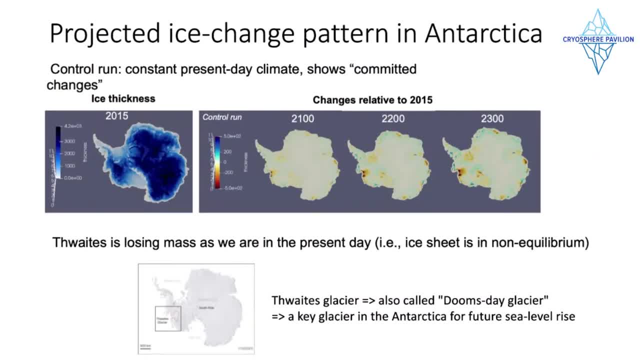 this results just looking at the spatial this results just looking at the spatial pattern of changes in the control run. pattern of changes in the control run, pattern of changes in the control run where we keep the climate change, where we keep the climate change, where we keep the climate change zero, so keeping the present day climate. 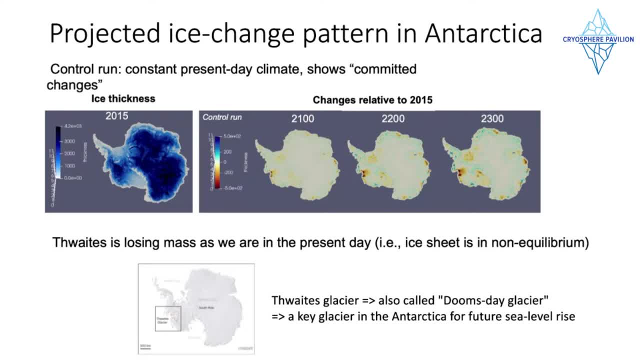 zero, so keeping the present day climate. zero, so keeping the present day climate. and yet we can see that the change is, and yet we can see that the change is. and yet we can see that the change is on the right hand side at 21st, on the right hand side at 21st. 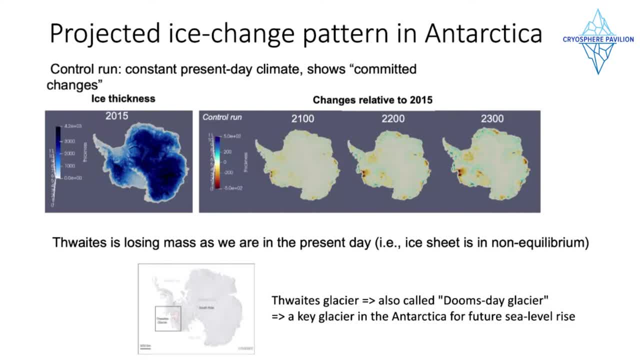 on the right hand side at 21st: 20- 2100- year 2200 and year 2300, 20- 2100- year 2200 and year 2300, 20- 2100- year 2200 and year 2300. there is still loss going on, shown in. 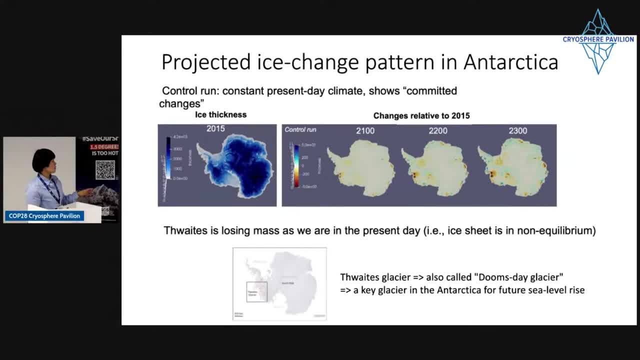 there is still loss going on, shown in. there is still loss going on shown in brown and yellow regions, specifically brown and yellow regions, specifically brown and yellow regions, specifically focusing on the west antarctic region, focusing on the west antarctic region, focusing on the west antarctic region. so that's, that's where the thwaites. 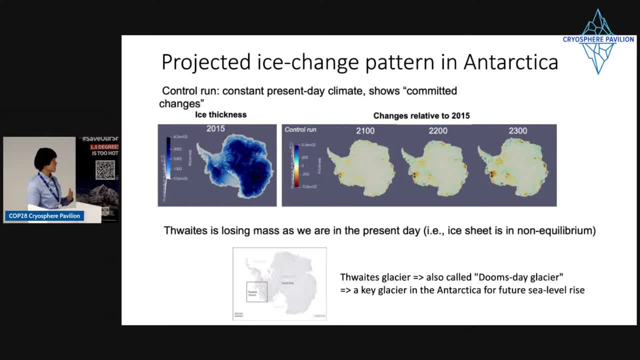 so that's that's where the thwaites. so that's that's where the thwaites. glacier, or so-called doomsday glacier, or so-called doomsday glacier, or so-called doomsday doomsday glacier, is glacier, is glacier, is um located, and this is really the key. 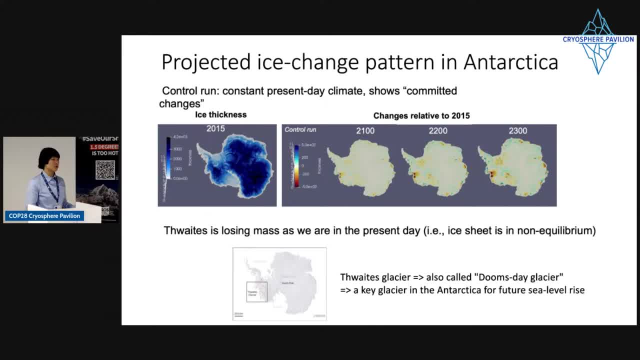 um located and this is really the key um located and this is really the key glacier in antarctica right now, that glacier in antarctica right now, that glacier in antarctica right now that everyone's concerned about, everyone's concerned about, everyone's concerned about for. 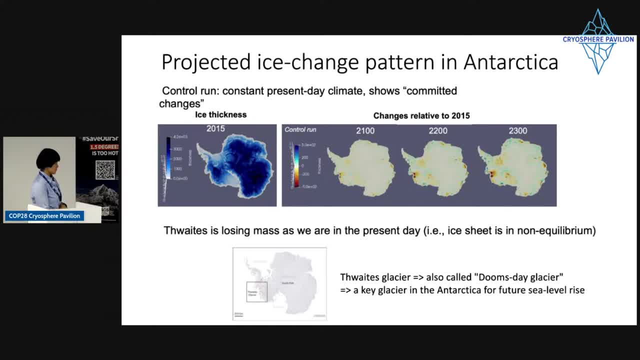 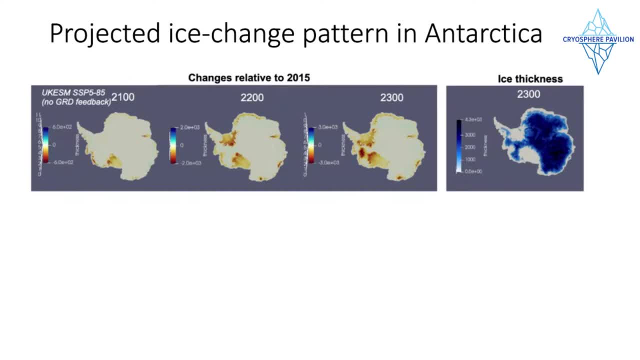 for for potential contributor to potential contributor to potential contributor to future sea level rise, and so i'm just picking the very high end. and so i'm just picking the very high end and so i'm just picking the very high end scenario: the uk esm ssb 5. 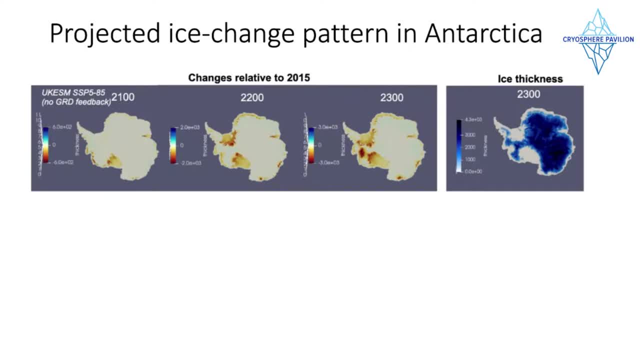 scenario: the uk esm ssb 5 scenario: the uk esm ssb 5- 8.5 forcing, where we've seen this 8.5 forcing, where we've seen this 8.5 forcing, where we've seen this really more than two meters of sea. 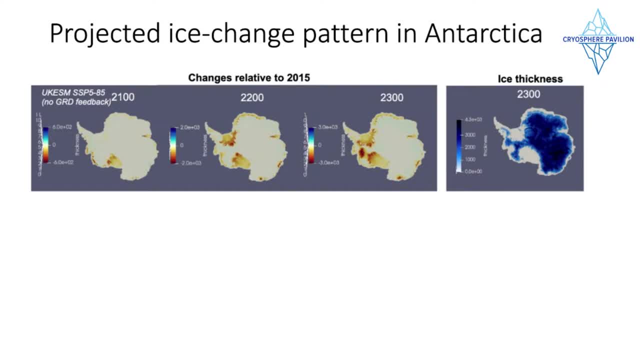 really more than two meters of sea, really more than two meters of sea level rise, level rise, level rise and the strong sea level feedback. and the strong sea level feedback and the strong sea level feedback effects, effects, effects. the plots here on the left show the. the plots here on the left show the. 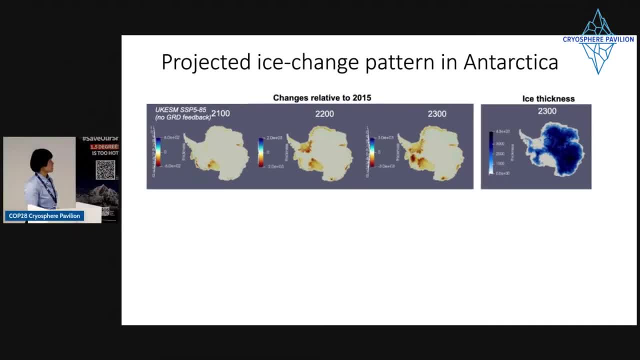 the plots here on the left show the changes: relative changes in ice changes. relative changes in ice changes. relative changes in ice thickness relative to 2015. thickness relative to 2015. thickness relative to 2015 at 2100, 2200 and 2300. 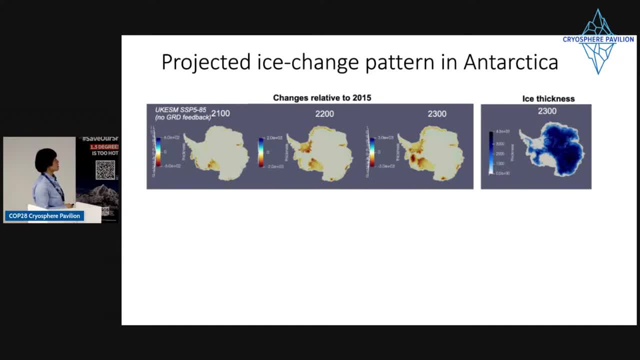 at 2100, 2200 and 2300, at 2100, 2200 and 2300, and then the final ice thickness at, and then the final ice thickness at, and then the final ice thickness at, 2300, 2300, 2300. you can see that all the ice shelves. 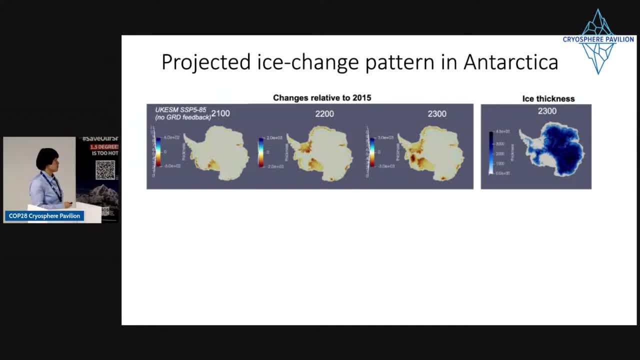 you can see that all the ice shelves, you can see that all the ice shelves were floating ice in the filch noroni were floating ice in the filch noroni were floating ice in the filch noroni and rossi and rossi and rossi ice shelf really all go away and also. 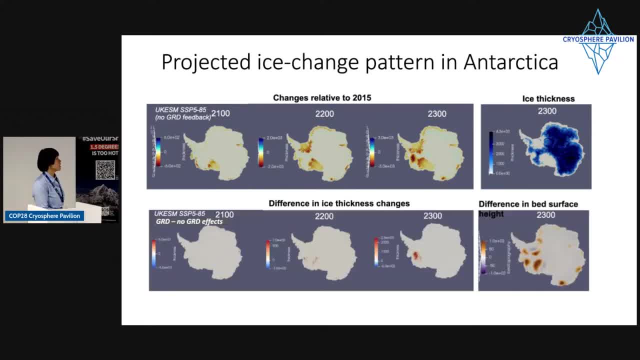 ice shelf really all go away. and also ice shelf really all go away. and also same for the western tardigate sheet, in same for the western tardigate sheet, in same for the western tardigate sheet in the thwaites region and and and the difference in ice thickness changes. 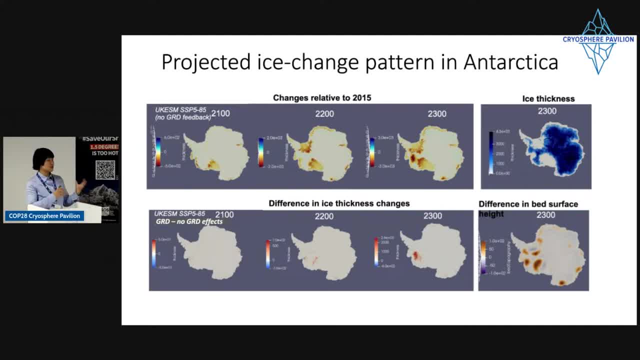 the difference in ice thickness changes. the difference in ice thickness changes when we incorporate the grd effects. when we incorporate the grd effects, when we incorporate the grd effects versus not not incorporating grd effects, versus not not incorporating grd effects versus not not incorporating grd effects, we can see that these effects last long. 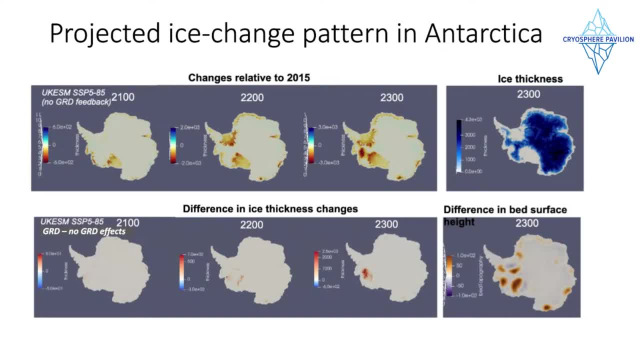 we can see that these effects last long. we can see that these effects last long, and by the end of and by the end of and by the end of 2300, there's a lot more ice surviving. 2300: there's a lot more ice surviving. 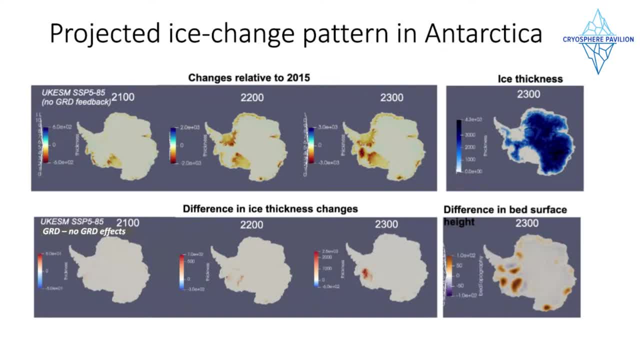 2300. there's a lot more ice surviving in the fifth region shown in red, in the fifth region shown in red, in the fifth region shown in red, right here, right here, right here. and that is again going back to this, and that is again going back to this. 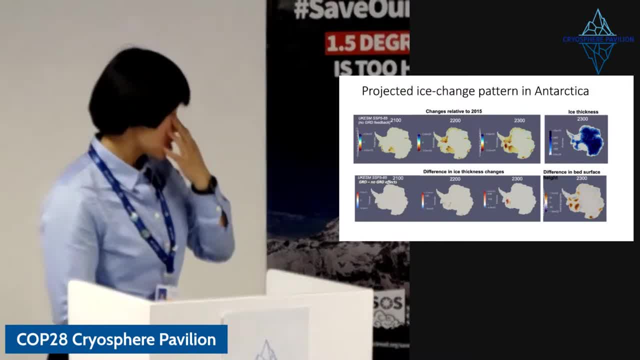 and that is again going back to this sea level fall or deformation grd effects. sea level fall or deformation grd effects. sea level fall or deformation grd effects shown in, shown in, shown in this spot, right here where the brown, this spot, right here where the brown, this spot, right here where the brown regions are showing where the sea level. 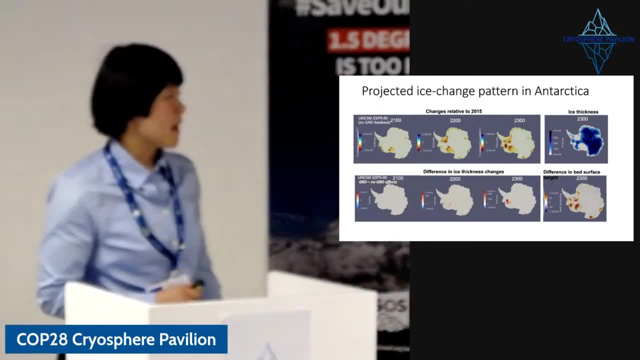 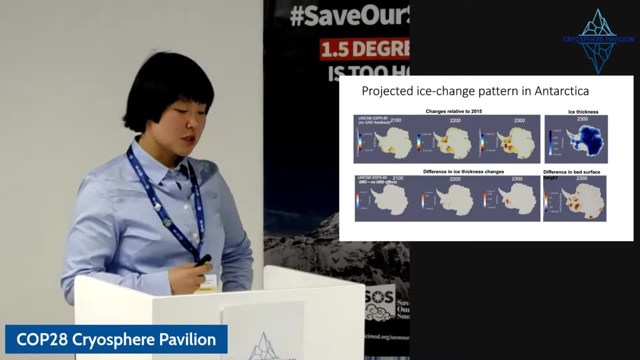 regions are showing where the sea level. regions are showing where the sea level, where sea level has fallen, where sea level has fallen, where sea level has fallen more than more than more than when we don't incorporate grd effects, when we don't incorporate grd effects, when we don't incorporate grd effects. so this, this plot, is really to show this. 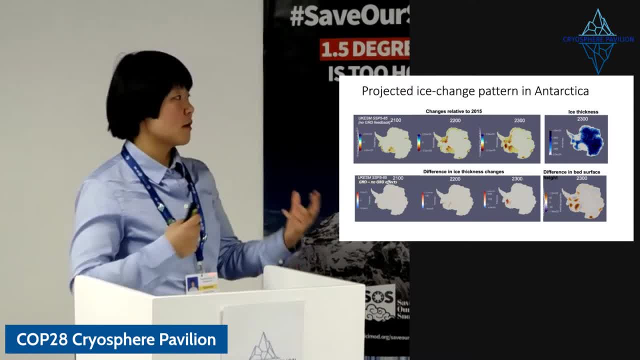 so this, this plot is really to show this. so this, this plot is really to show this: how the feedback capturing the feedback, how the feedback capturing the feedback, how the feedback capturing the feedback provided capturing feedback of grd. provided capturing feedback of grd. provided capturing feedback of grd- effects. 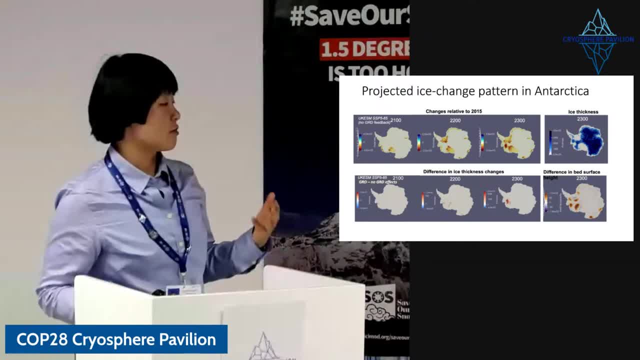 effects, effects in our ice sheet projections, in our ice sheet projections, in our ice sheet projections change our projections by much, change our projections by much, change our projections by much. um and um and um, and those, those, those huge differences in ice thickness. huge differences in ice thickness. 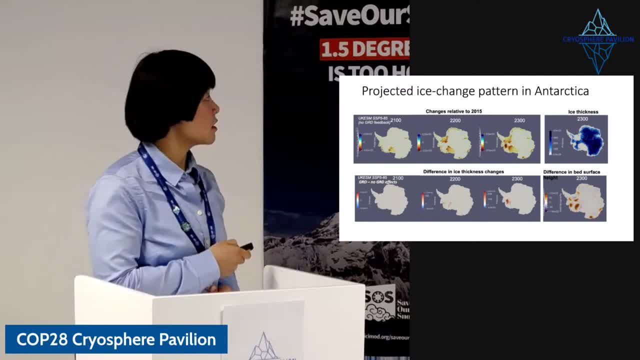 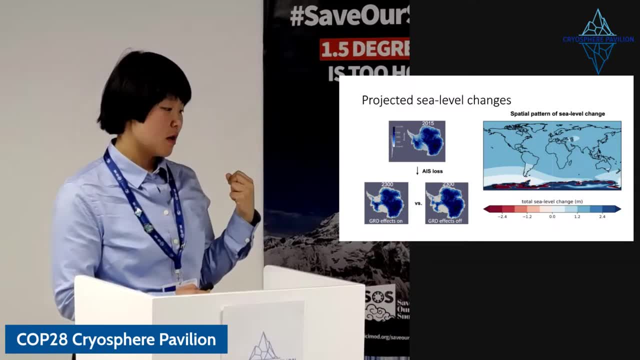 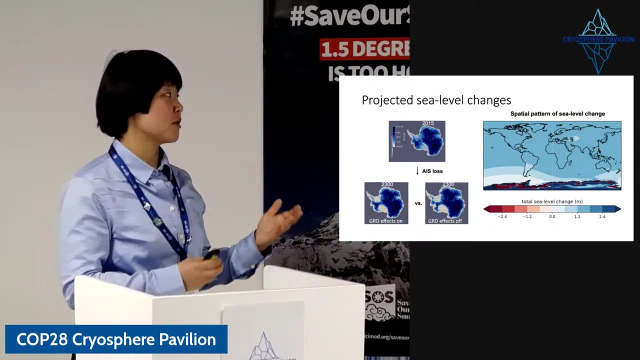 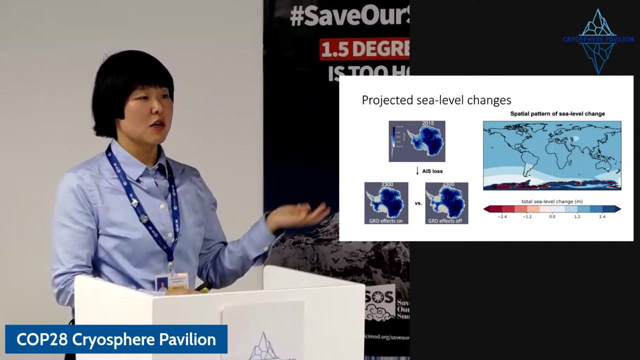 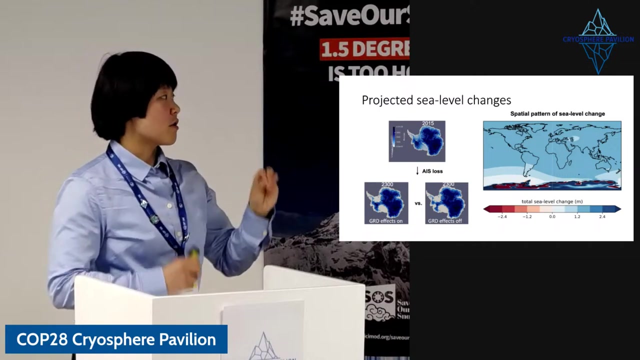 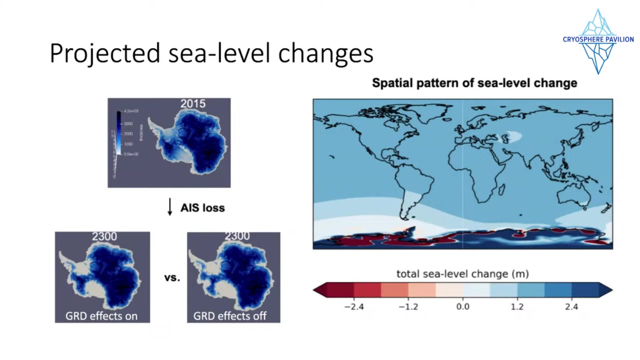 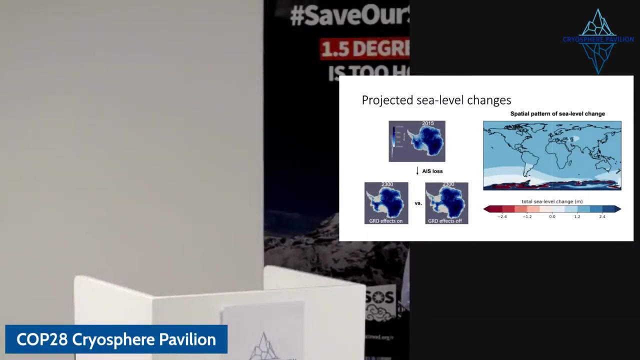 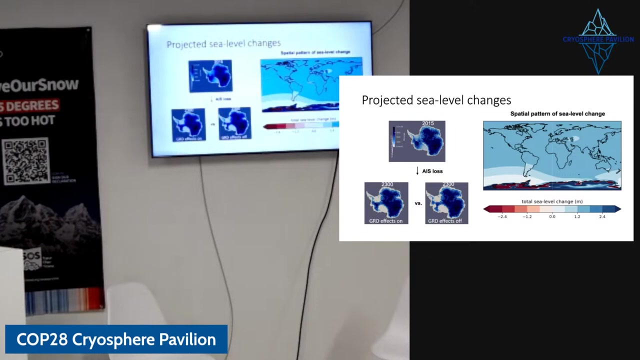 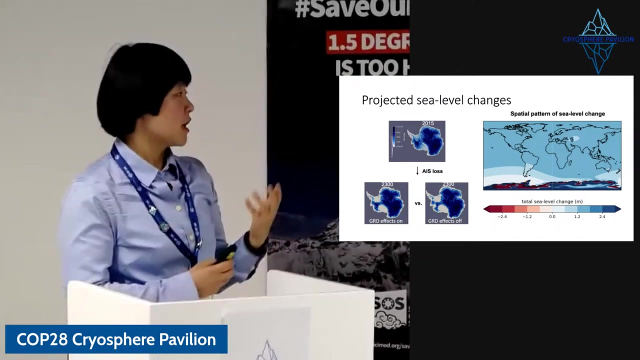 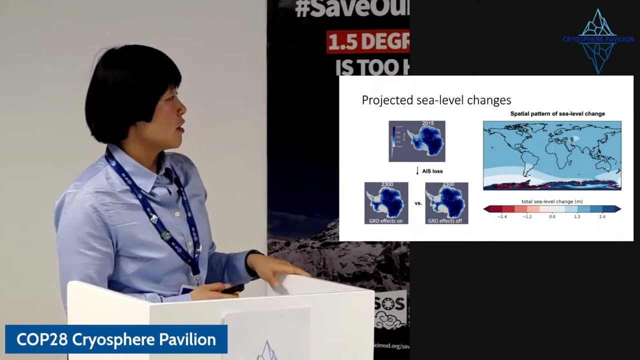 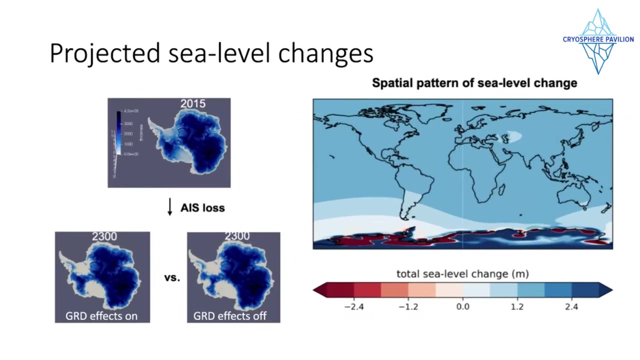 huge differences in ice thickness, especially in the region of our interest, especially in the region of our interest, especially in the region of our interest at the moment. so so, um more than globally, i mean a. um more than globally, i mean a. um more than globally, i mean a globally averaged value. 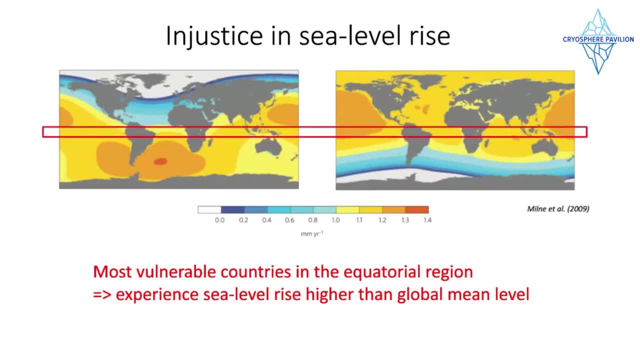 globally averaged value. globally averaged value. so, so, so, um, i just wanted to go back to the point. um. i just wanted to go back to the point. um, i just wanted to go back to the point where, where, where, or bring up a point where, or bring up a point where. 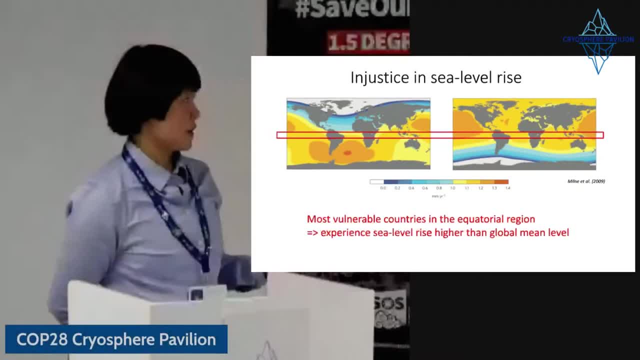 or bring up a point where i'm doing this climate science or this, i'm doing this climate science or this, i'm doing this climate science, or this topic of research of my interest, but topic of research of my interest, but topic of research of my interest, but also i'm more motivated to continue. 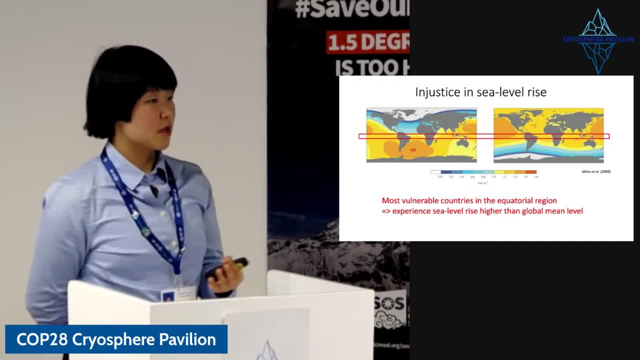 also, i'm more motivated to continue. also, i'm more motivated to continue this research because this research, because this research, because it's not only about understanding, it's not only about understanding, it's not only about understanding physical processes, but it was also physical processes, but it was also 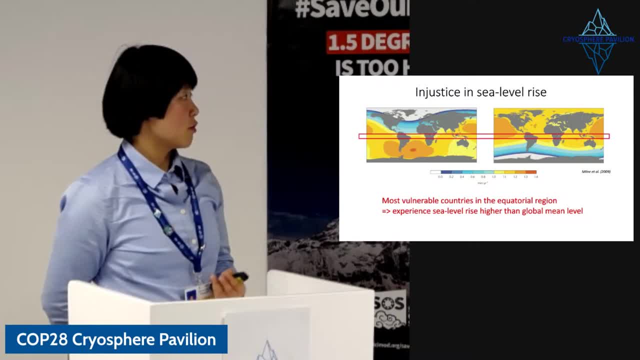 physical processes, but it was also about understanding, about understanding, about understanding um our world in a more um our world, in a more um our world, in a more humanity, humanistic way, humanity, humanistic way, humanity, humanistic way, so to speak. this is really showing, so to speak. this is really showing 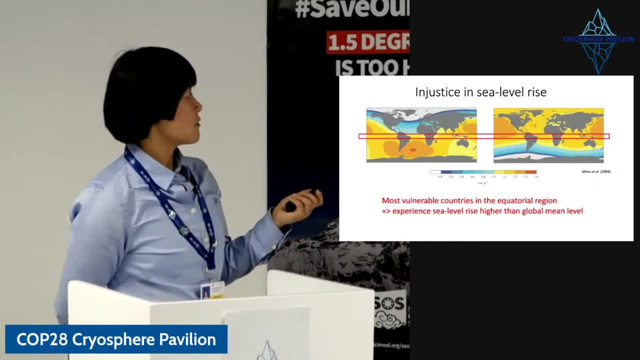 so to speak. this is really showing that, regardless of that, regardless of that, regardless of where you melt the ice from, either from where you melt the ice from, either from where you melt the ice from: either from the northern hemisphere or from the- the northern hemisphere or from the. 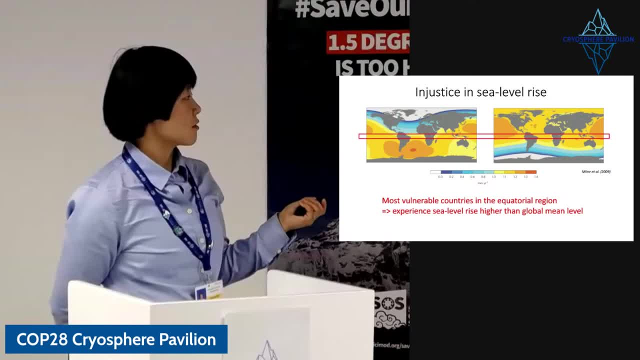 the northern hemisphere or from the antarctica, antarctica, antarctica, the most vulnerable countries in the, the most vulnerable countries in the, the most vulnerable countries in the equator, equator, equator countries, to sea level rise is in situated in the equatorial region and so situated in the equatorial region and so situated in the equatorial region, and so they are going to experience sea level. they are going to experience sea level. they are going to experience sea level rise higher than global mean sea level rise higher than global mean sea level. 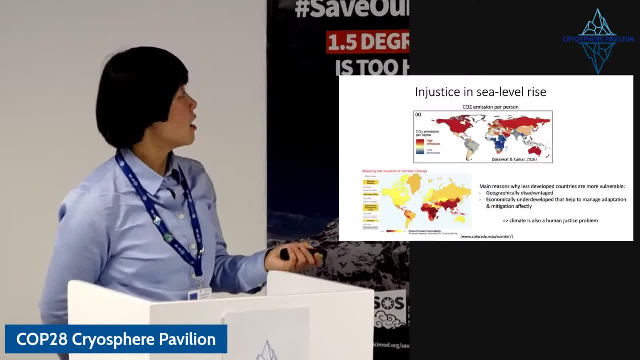 rise higher than global mean sea level. regardless, regardless, regardless of where we melt is from, of where we melt is from, of where we melt is from, and just showing the co2 emission per. and just showing the co2 emission per. and just showing the co2 emission per person. 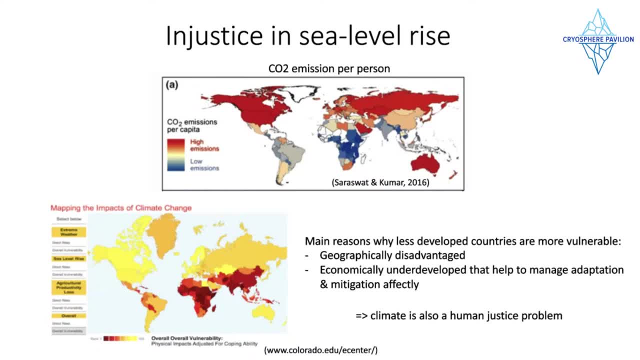 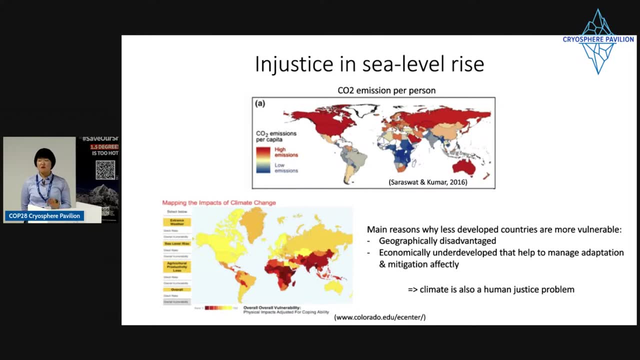 person, person around the globe, these equatorial regions around the globe, these equatorial regions around the globe, these equatorial regions, these countries have contributed almost. these countries have contributed almost. these countries have contributed almost nothing, um nothing, um nothing, um. i was talking to a jamaican seaweed. 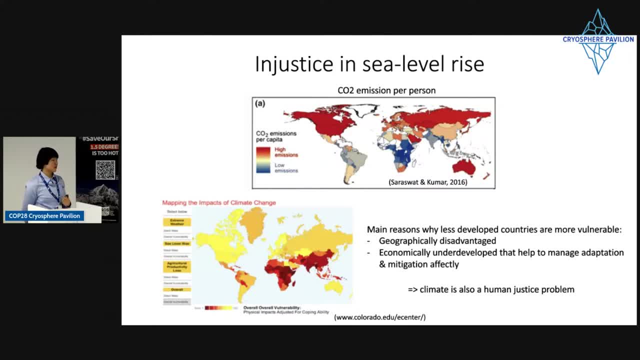 i was talking to a jamaican seaweed. i was talking to a jamaican seaweed farmer yesterday at the cryospheric farmer, yesterday at the cryospheric farmer, yesterday at the cryospheric pavilion, and he was really pavilion and he was really 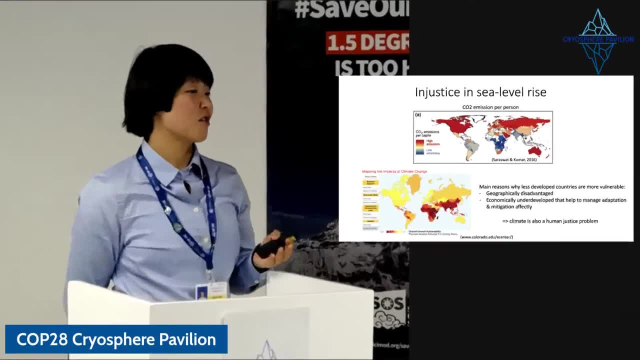 pavilion and he was really concerned and he was bringing up the concerned. and he was bringing up the concerned and he was bringing up the point where his country point, where his country point, where his country contributed about 0.04 percent of the contributed about 0.04 percent of the. 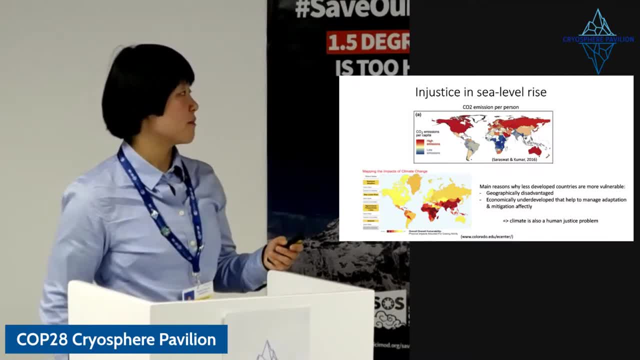 contributed about 0.04 percent of the total co2 emission. total co2 emission. total co2 emission, co2 emitted co2 emitted. co2 emitted in the world, in the world, in the world. so so, so, yeah, just bringing the human humanity. yeah, just bringing the human humanity. 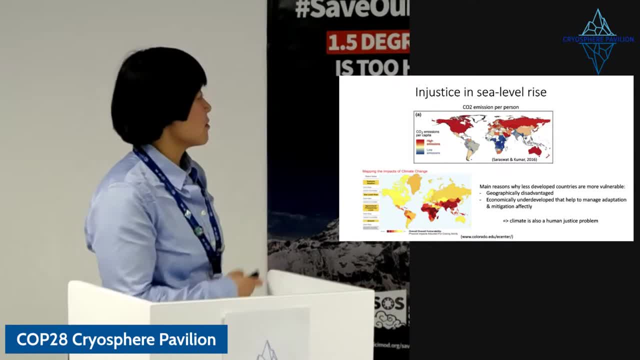 yeah, just bringing the human humanity point of view point of view, point of view um to research, and then the bottom plot um to research, and then the bottom plot um to research, and then the bottom plot shows shows: shows the impacts of climate change around the. the impacts of climate change around the. 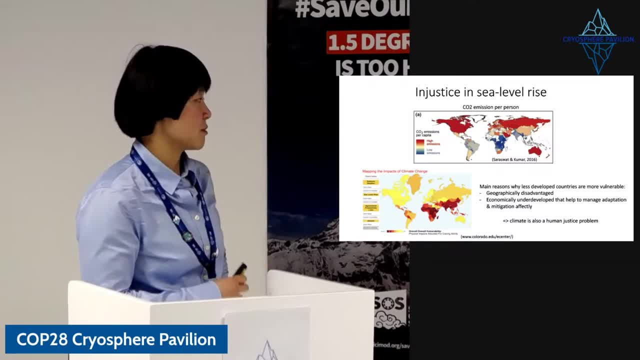 the impacts of climate change around the world, and the red plot is world. and the red plot is world. and the red plot is red. regions are where it's more, red regions are where it's more red regions are where it's more vulnerable, vulnerable- vulnerable to climate change- and we can really see. 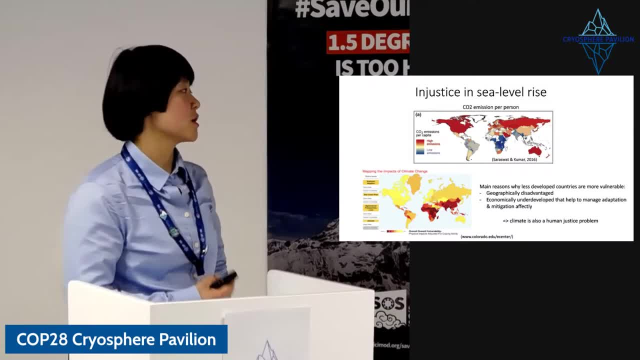 to climate change and we can really see to climate change and we can really see that, that that these regions are where they're less. these regions are where they're less, these regions are where they're less developed, developed, developed and the main reasons why these less and the main reasons why these less. and the main reasons why these less developed countries are developed countries are. developed countries are more vulnerable to sea level rise and more vulnerable to sea level rise and more vulnerable to sea level rise and climate change in overall is because climate change in overall is because climate change in overall is because they're not only geographically. 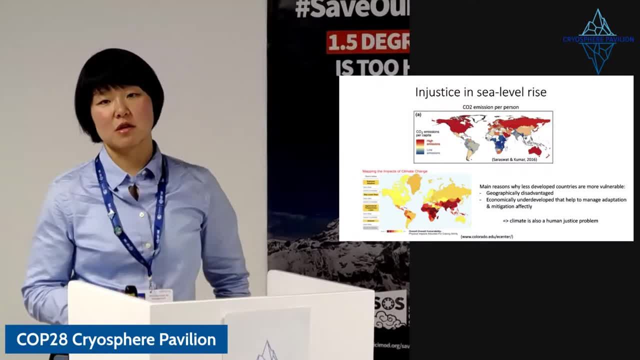 they're not only geographically. they're not only geographically disadvantaged, but also they're disadvantaged, but also. they're disadvantaged but also. they're currently economically underdeveloped, currently economically underdeveloped, currently economically underdeveloped. so they are more so, they are more so, they are more. yeah, they can't really manage the.